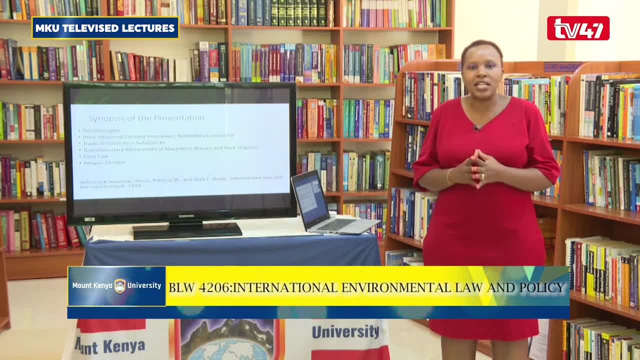 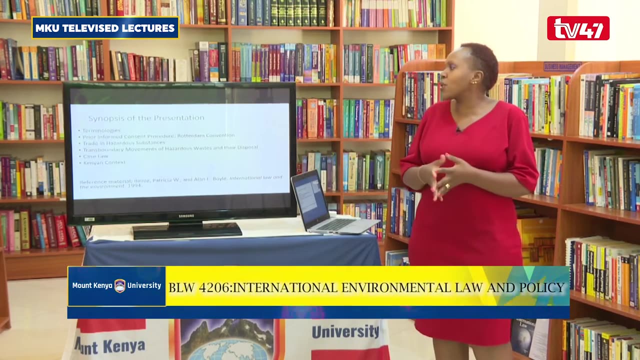 for example, if uganda wants to transit hazardous toxic substances to kenya- and we know there's a country perhaps in between, so we must get prior consent from uganda- any country that the goods, that the goods will be passing through, and kenya also as a recipient country. we look at a few case. 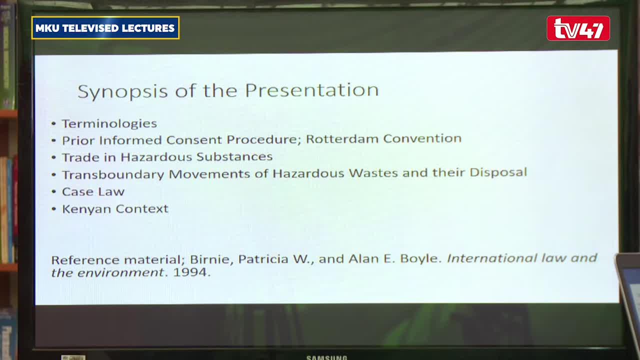 laws, basically looking at the emergence of the need to come up with a low regulatory framework on hazardous and toxic substances, basically laws, the case, the incidences that happen before some of these laws that we'll be discussing were developed. then we finalize our discussion with the kenyan context. what does the law say in kenya? what provisions do we have? institutional framework: 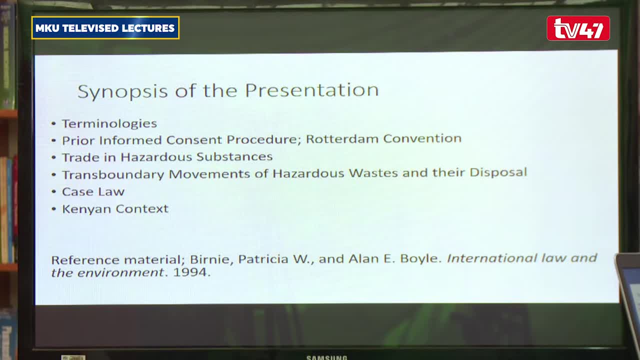 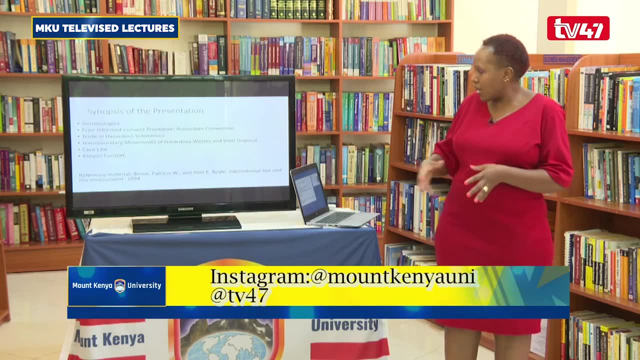 do we have in terms of management of waste products in our country? one of the reference key material that we've been discussing in all previous classes is the book by bani and patricia, which is basically international law and environment 1994.. so kindly remember, as we normally refer to that textbook, that is our lead textbook, which has 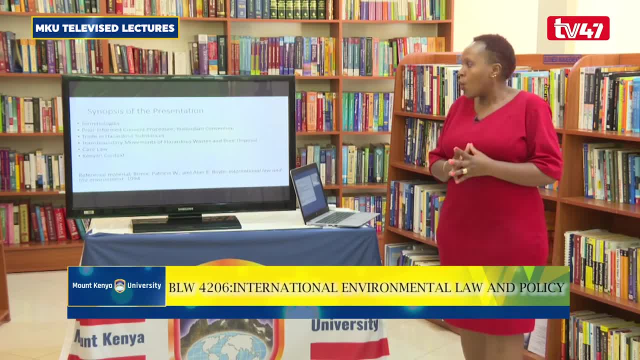 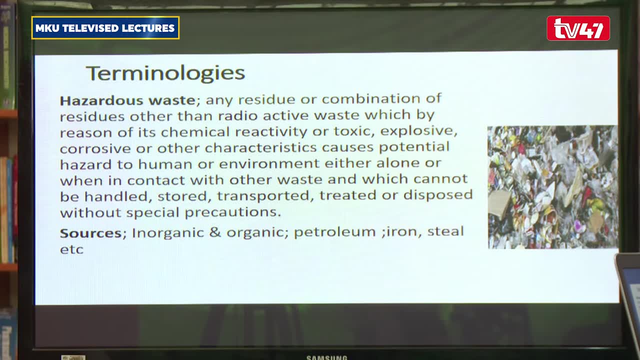 been available in the library, but you can also get a version of it online when you utilize the different platforms that you have at the university. so i will commence by discussing what is hazardous waste products. basically, these are residues or combination of residues from chemical products. these are waste products. they might be organic or inorganic. 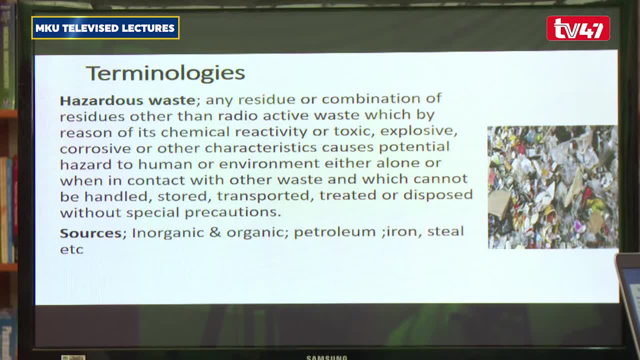 but basically a product that if they are not basically managed properly, they are harmful to the environment and they are harmful for human beings. it might be corrosive. for example, you can find an acid waste product that when it touches your skin it corrodes with your skin or when it is inhaled. 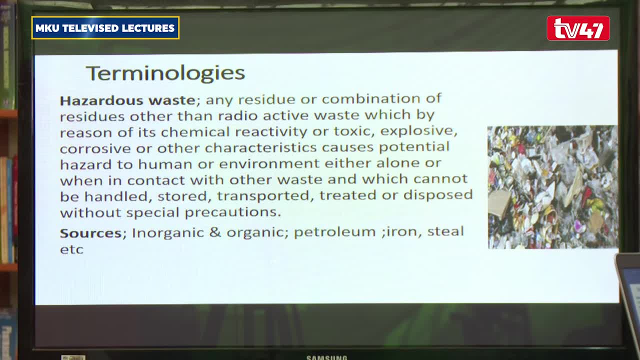 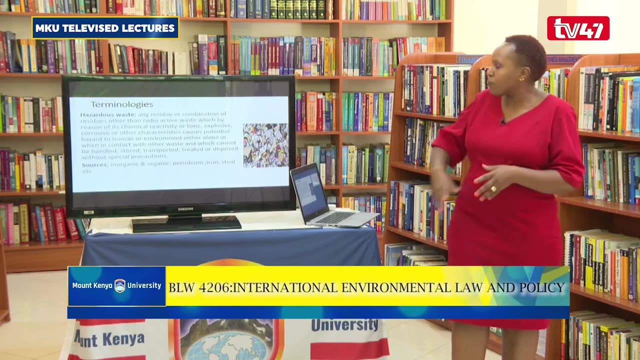 for example, when you're spraying doom in your rooms and you inhale that doom to a higher concentration or you omit it to a level that is harmful to your health, it will lead to inhalation of toxic substances, substances which will deteriorate your health, your health generally. there are other hazardous. 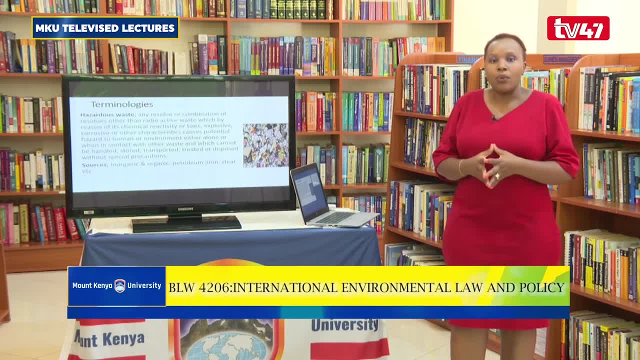 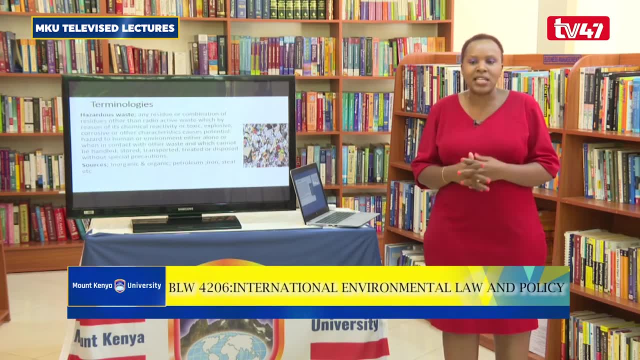 waste products that are explosive. when we dispose of and discard our waste products in the house, it's normally recommended- and it happens more in developed countries- that the waste product that is organic is where is managed separately from inorganic product. for example, you can't dispose of a doom, a container which had doom, or pesticide with cabbages and potatoes that. 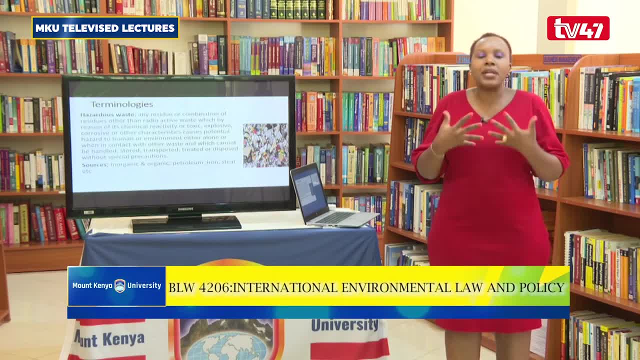 use as a byproduct, because that mixture also brings another level of toxics and hazardous substances that might be harmful to the environment outside there, but it also be harmful in your internal environment in the house. so that you are looking at how do you manage these substances to for our own protection in our household level. 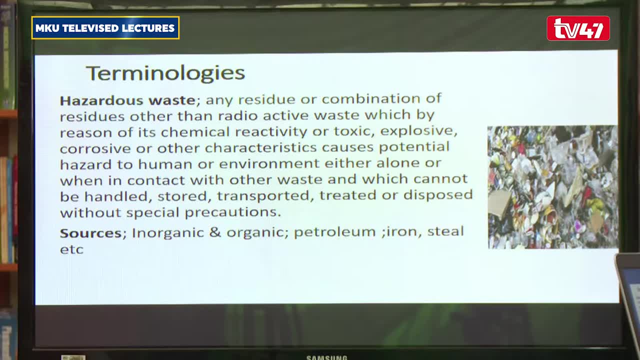 but the protection of the global environment, because we are the users, we are the ones who mix these chemicals to be able to produce a material that we need. in some instances, we mix them that it level that it comes the radioactive material which has nucleolites we've. 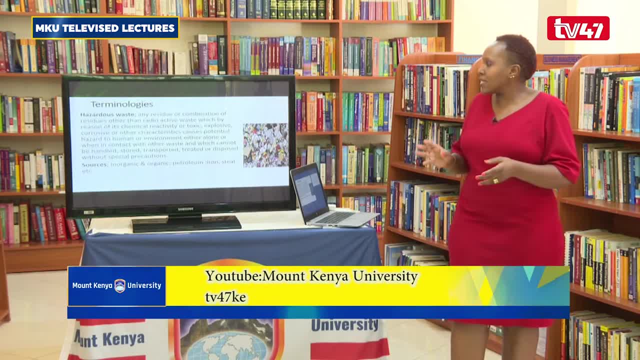 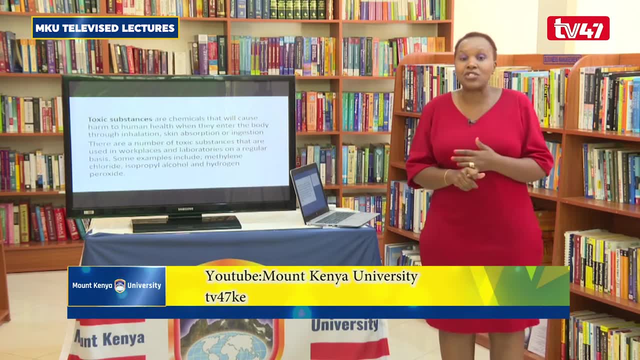 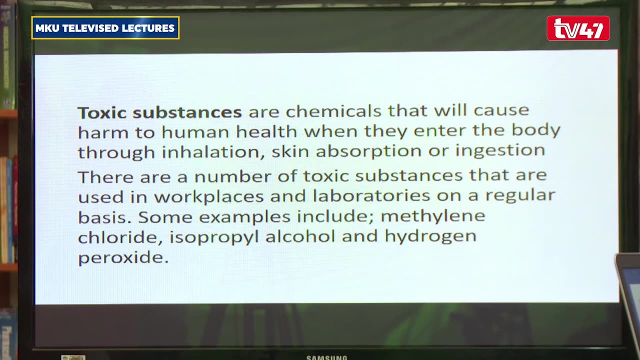 been discussing this in the in previous classes. so why it is important for us to manage this product is because we don't have a clear infrastructure- the global level- on management of as ideas and waste product. then we also lack sufficient regulatory and institutional frameworks at country level to manage. 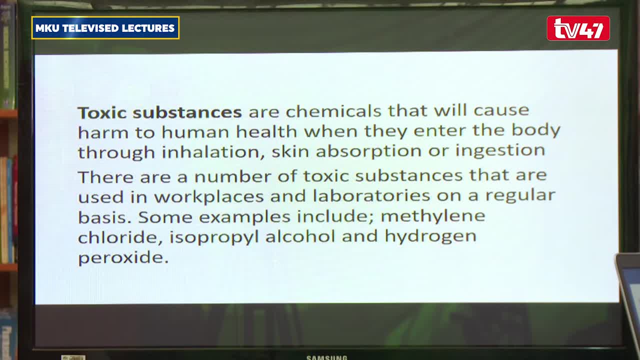 waste management products can go to Kenya, we have NEMA, the National Environmental Management Authority- but in other countries this is a discussion that they have to put it in their top agenda. toxic substances are a component of hazardous substances. they're toxic because these are chemicals. they are. 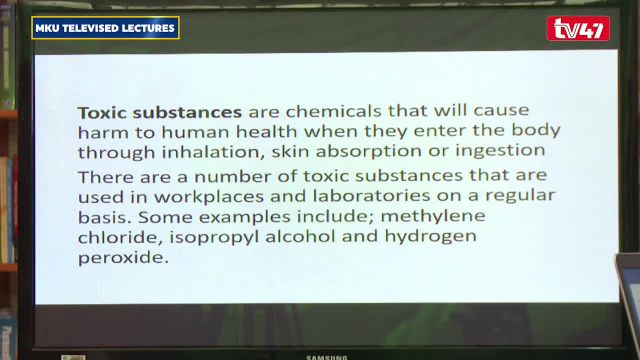 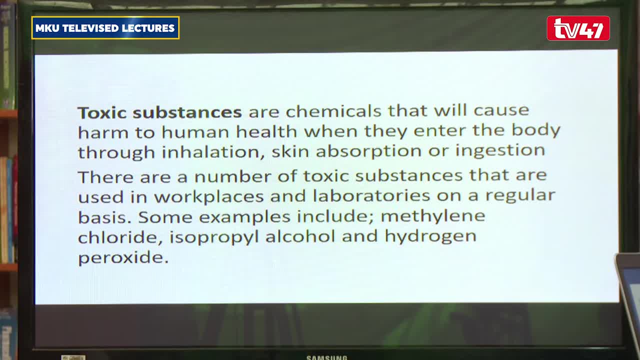 for human beings, for the survival of human beings. we can make reference even to the current situation that you have of coronavirus COVID-19. we are not so sure of the substances that were mixed for us to be able to now experience environmental damage. human beings are fighting for survival because of a 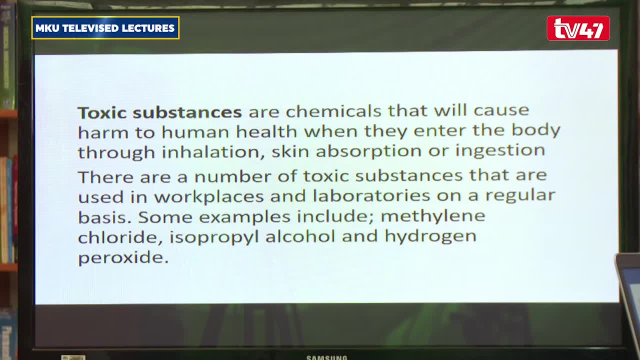 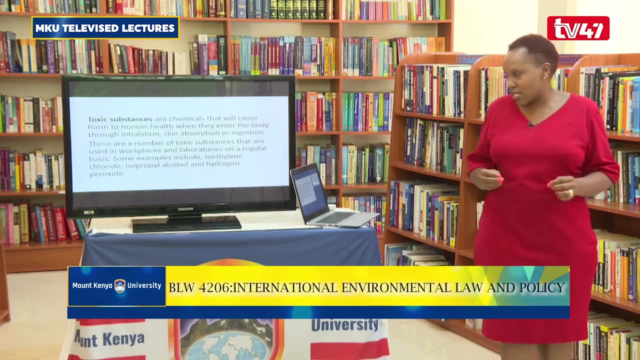 chemical reaction that was mixed up that is now a byproduct of a process that is harmful to the environment. these are the current discussions that you are looking at, and these are the issues that inform why we need to look carefully on the trade in hazardous and toxic substances at the global level and as international. 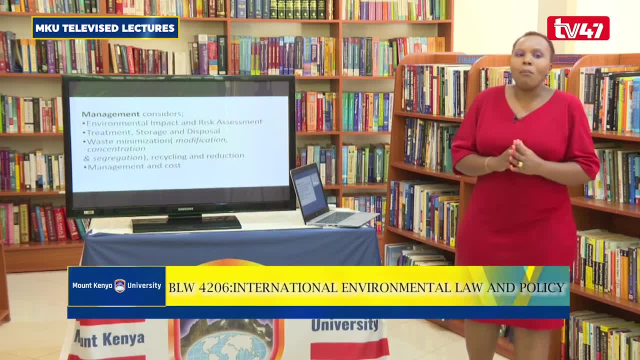 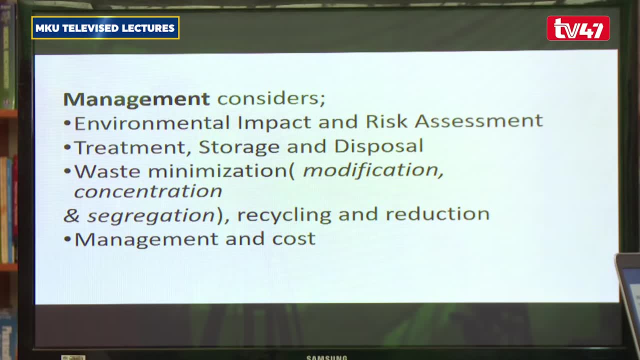 and at the national level. so, management: why we need to manage them? one is because we want to see what is the impact, the risk assessment, of us having a nuclear plant in Kenya, what happens when there's an incident or leakage of new radioactive materials from these nuclear plants. this is why we need management at 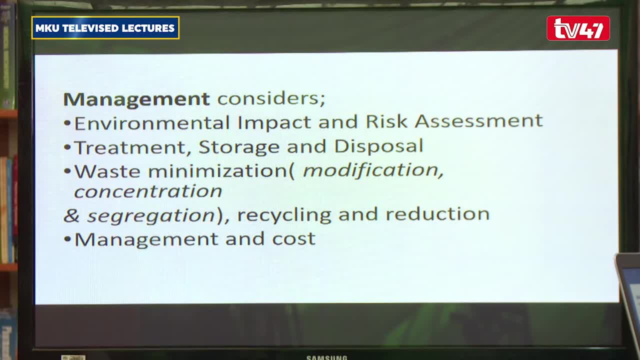 the global level. we need to adhere to guidelines at the global level and at the national level. how do we treat and store this waste products if we permit a country, to an industry to develop, to install a nuclear plant, for us to be able to have lights, for us to be able to have batteries to charge our, our phones? 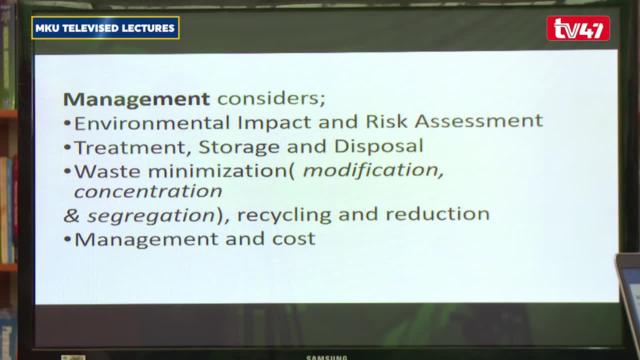 batteries to charge our radios and touch. we must look at what is the storage mechanism for this product. when you have a pro, you want, at the end of the day, to produce a battery. why do you manage the waste products that come from that production of the battery? that is the problem that you want to address in our 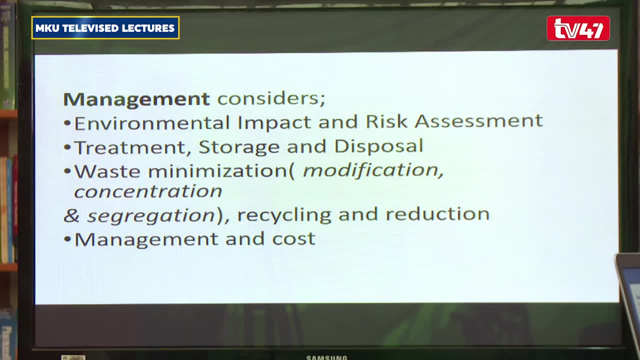 today's class, the disposal mechanism. what are the disposal mechanism within your country or context that are favorable enough to ensure that there is no leakage, there's no exposure to the environment of this toxic cell as other substances? there are countries who come up with a sink. they basically dig a big. 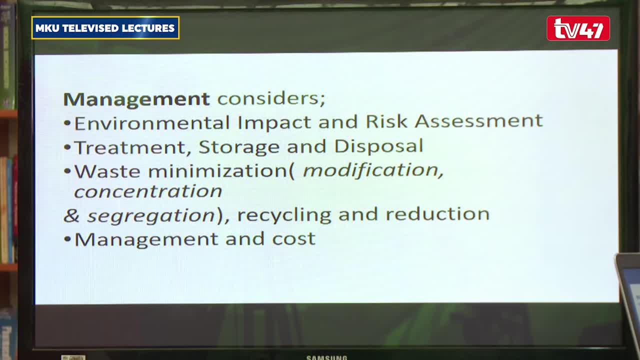 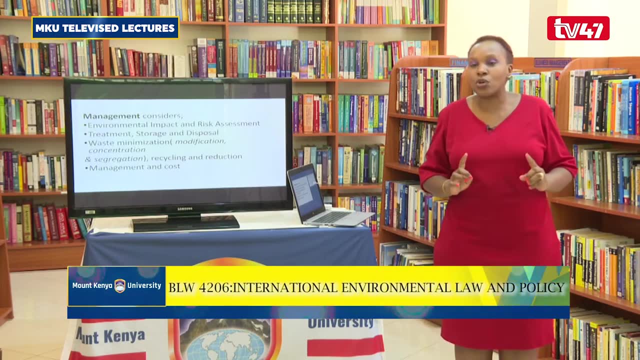 hole, they construct a sink made of metal to be able to build a battery, to produce a battery, to produce a battery that is, dump and store all those waste products so that they are not exposed to the environment. but remember, in our previous this class, we also discussed how you can. 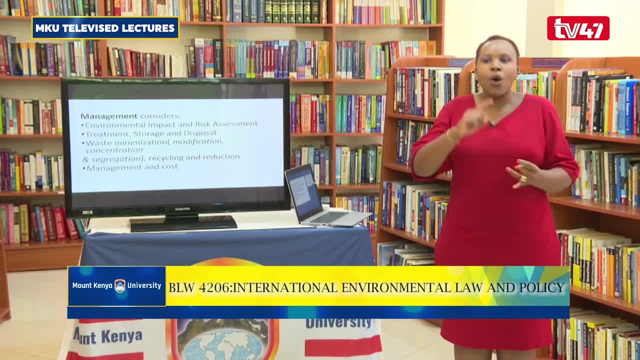 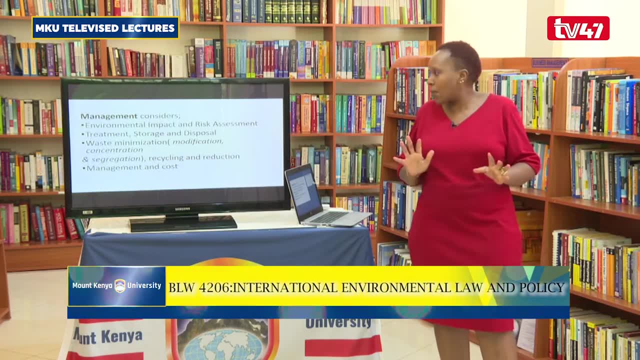 construct a sink, you need approval from the conference of parties. when you're opening your sink, you also need approval from the conference of parties. but basically that is what one of the mechanisms are using in waste management. the other aspect of it is waste minimization because, remember, we produce. 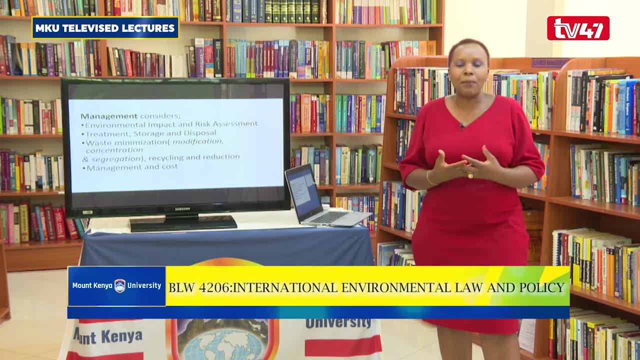 a product, but how you modify them. look at our Dandora dumping sites. Dandora dumping sites is a dumping site. yes, that is designed by the government for us to be able to dump our waste products. but how we dump them. we have modified the byproduct: cabbages mixed together. we do mix together with all other used products. 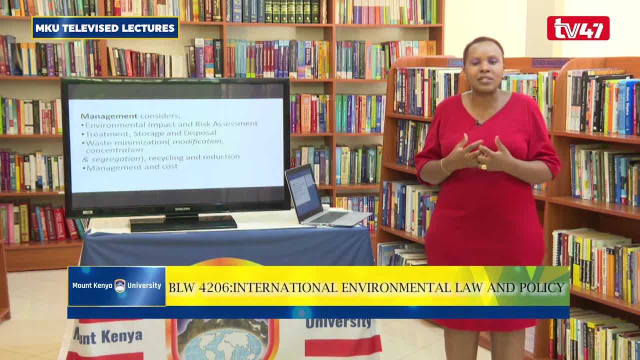 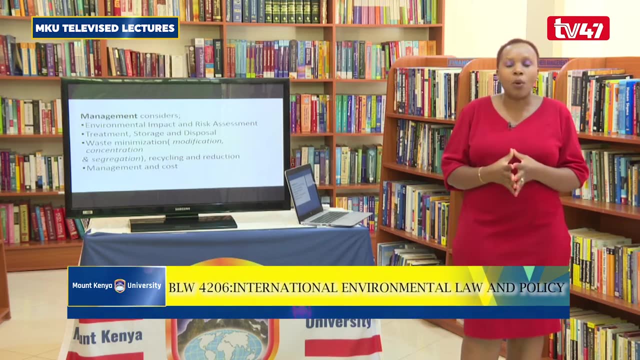 within our household that brings out a certain level of intoxication to the environment and to the community. these instances will have increased in the number of cancer cases in our country because of our poor management of waste products. the concentration level is also one of the key components that is important in terms of management of this products. 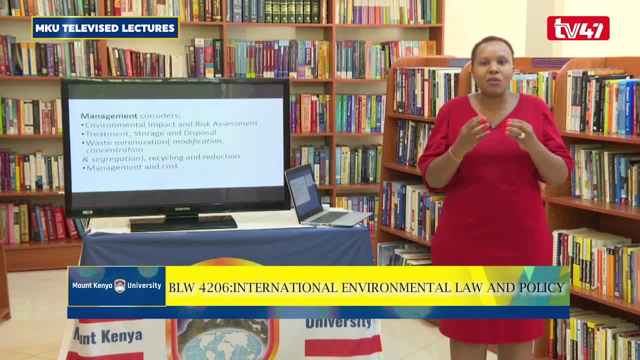 because the level of emission of these gases- some of them are gases, some of them are liquid, some of them in solid form- the level and capacity of emission of discusses gases is important and critical to the global level because, remember this, gases emit from the ground when we use them, or a fertilization, or even maybe the organic product that you're getting from the byproducts from animals. They come up, they mix with other gases into the air, they go to the ozone layer, mix with the ozone gas and, of course, they cause depletion of the ozone layer. This is one of the things that 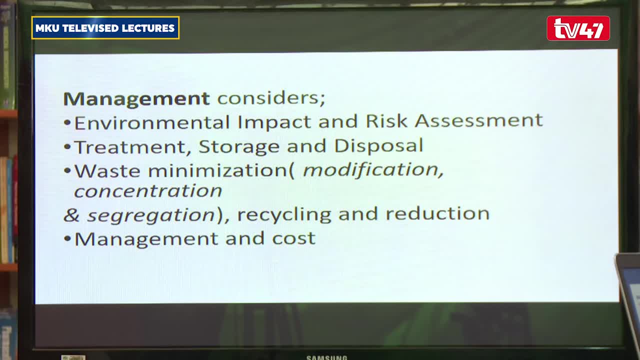 we need to protect at the global level is how this waste product contributes to the depletion of the ozone layer. We look at also another issue of management and cost. Why we need this regulation of azalea substances at the international level is for us to see how countries can be able to. 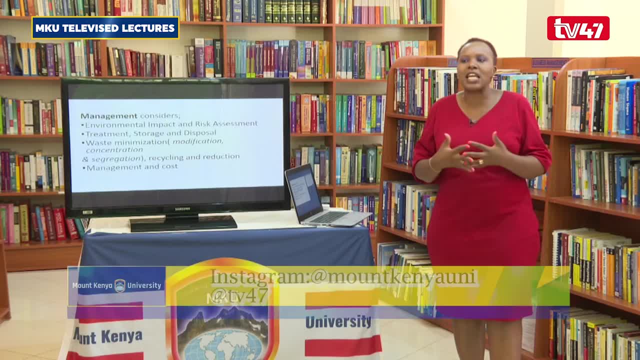 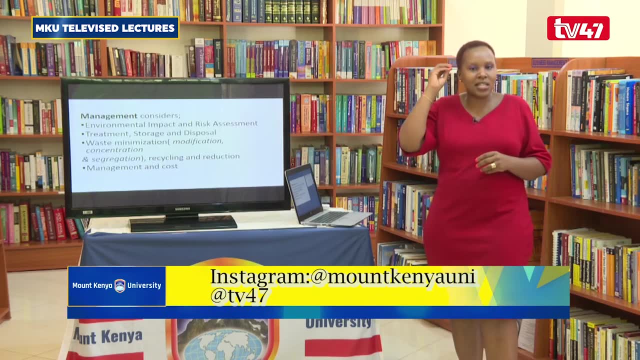 share the management of this product so that if your capacity level in terms of finances are a bit low- and we know that- if you're having an industry that produces waste products that are dangerous to the environment, at the end of the day, we need to consolidate all our funds to be able to address. 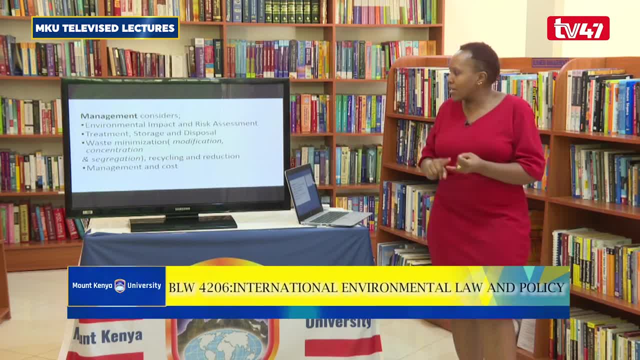 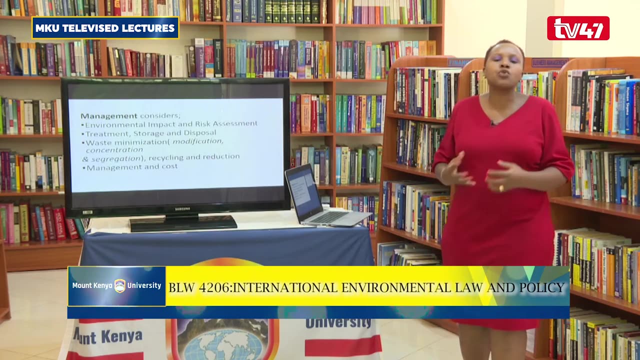 issues of protection of the ozone layer. That is where management and cost effectiveness must be done at the global level and see how we can support countries like Haiti. Haiti has been a victim of dumping of waste- Hazardous waste products- But Haiti does not have the financial capacity to dispose them. So we are coming up with a. 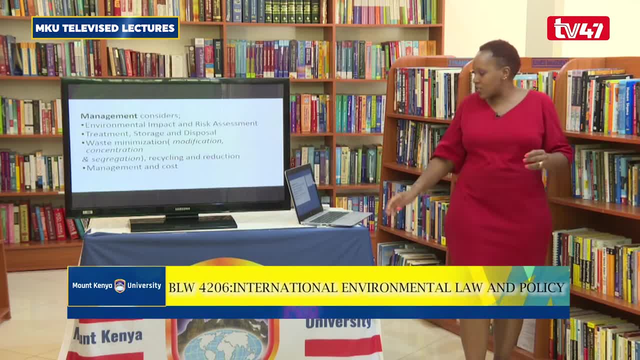 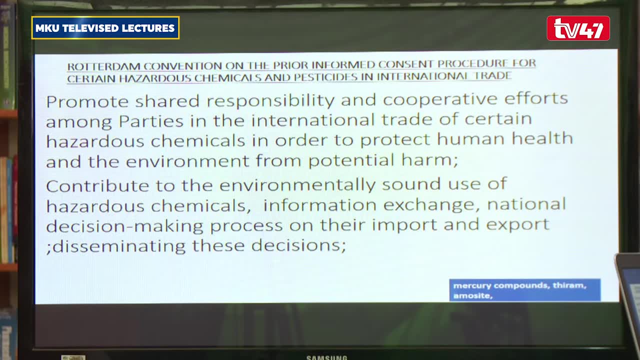 consolidated fund, the Green Fund, to be able to assist countries that do not have resources for that. So in that context, at the international level, we came up with a Rotterdam Convention on the prior informed consent procedure for certain hazardous chemicals and pesticides in international trade. Basically, this is referred to. 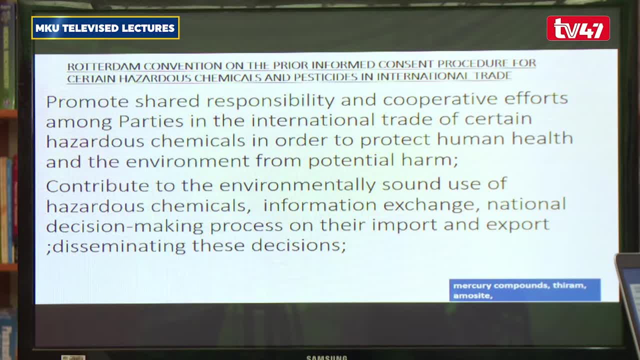 us as the Rotterdam Convention. It's a convention that emerged after the Rio Conference. Remember, in the first class we discussed about the Rio Conference. It gave us the Rio Declaration And one of the things that it gave us also is the Agenda 21.. So Article 19 of the 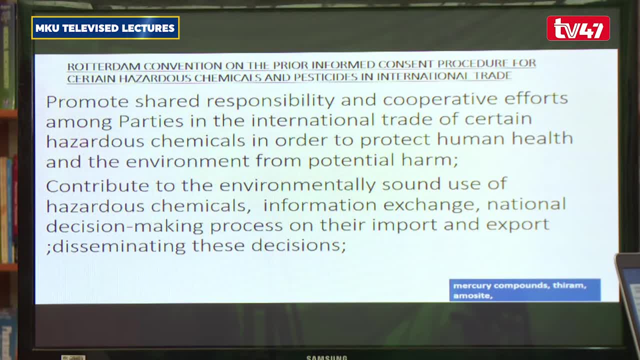 Agenda 21 talks about the need for countries to manage waste products that are dangerous to the environment and human health. This is why the case of the Rotterdam Convention was enacted: For it to be a global regulatory settlement for countries to be able to be bound with the procedures of regulating hazardous and toxic substances. But 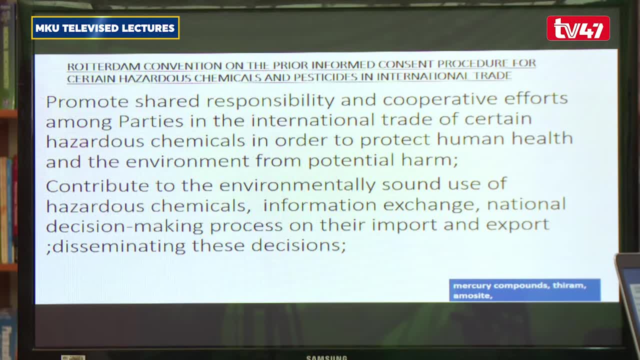 specifically. also, this Convention recognizes that we have the authority to do trade, but how do we do trade? that we ensure that we cover the countries that are not interested in trading hazardous and toxic substances. So one of the key responsibilities of this Convention- basically there are two- One is introduction of the principle of prior informed consent. 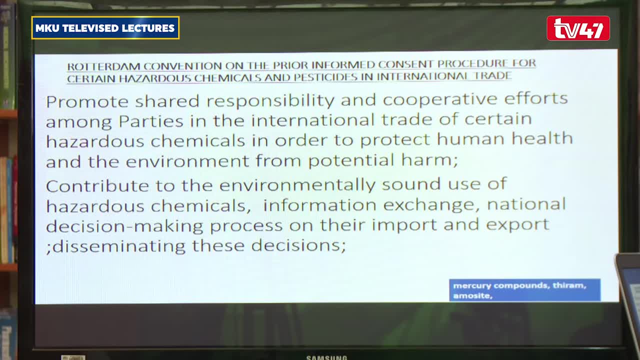 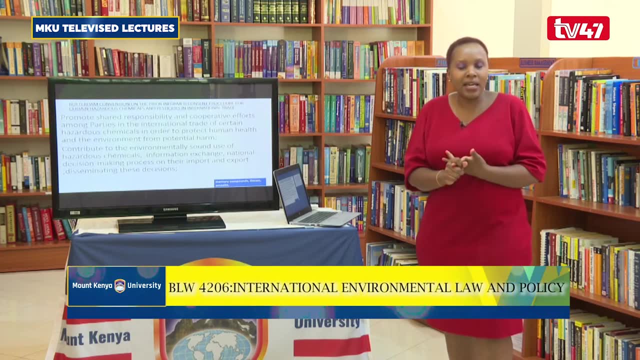 One is the introduction of the principle of prior informed consent. The other isn't incidental, but that's what we do Of. other one is the principle of information sharing, because why it is important is we had a case which is called the Kian case, K-H-I-A-N case, which is a 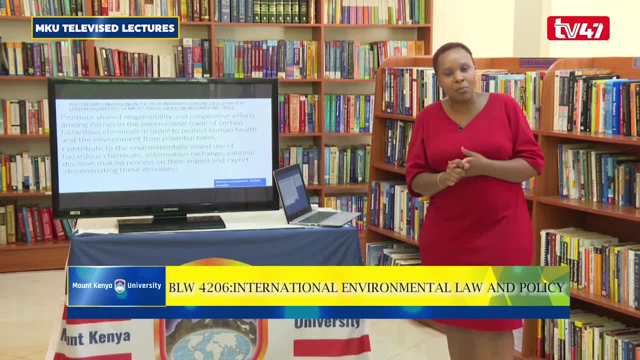 case of a company called Kian, which was established in Liberia. basically, what they did they? they attempted to dump waste product in a form of ashes in a New Jersey. they attempted to dump it in Bahamas. they attempted to dump it in Panama, but those countries refused. but at the end of the day, those ashes were. 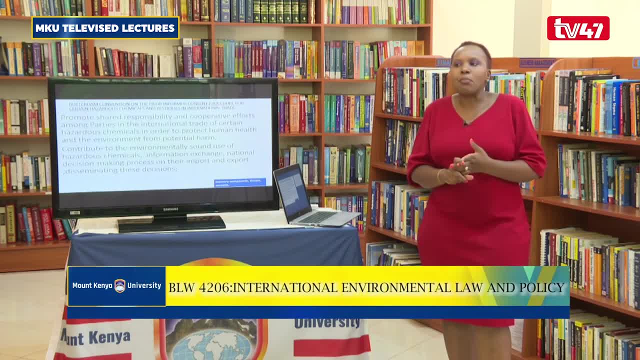 dumped in Haiti, which basically without approval of Haiti as a country, and once those products were dumped, it took Haiti. the products were dumped in 1988 but up to to date, as recent as 2000, Haiti was still working on disposal of those, management of those waste products that were dumped from from that company. they 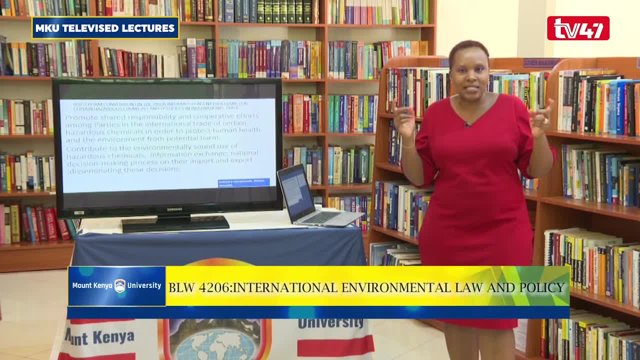 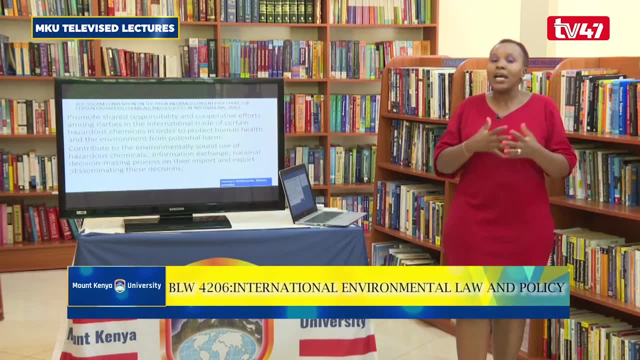 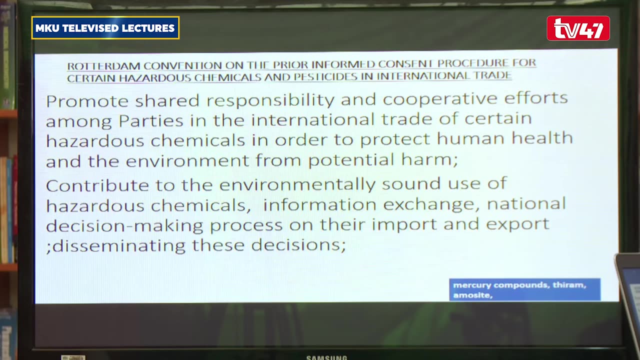 claimed they were dumping for fertilizer- topsoil fertilizer- so Haiti? well, the farmers in Haiti agreed to the dumping because they thought this, the topsoil fertilizer that is going to help the country in terms of the production. crop production basically turned out to be a hazardous and toxic substances in form of us. off course, the case was. 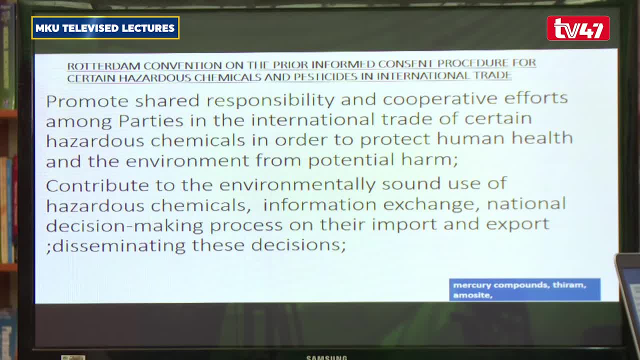 prosecuted and the country was head-luck. so these are the two principles that the convention is coming on board, because listen of shared and cooperative responsibilities between countries. the other is information sharing so that countries are aware about their council responsibilities, but the other one is information sharing so that countries are aware of the 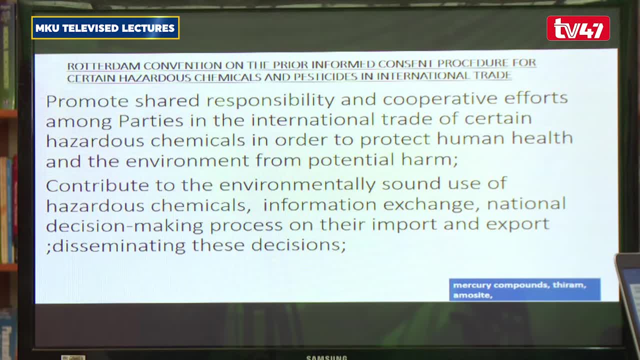 of who is doing trade if kenya and rwanda, for example, come up with an agreement to transfer to to trade in azeda's toxic substance or radioactive materials. so we know uganda is in the middle of kenya and and rwanda. so the informed consent as a principle in this 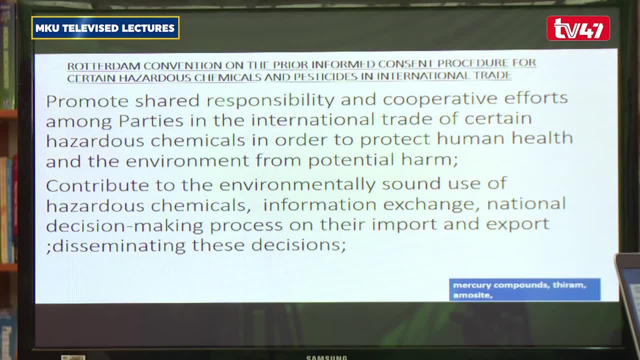 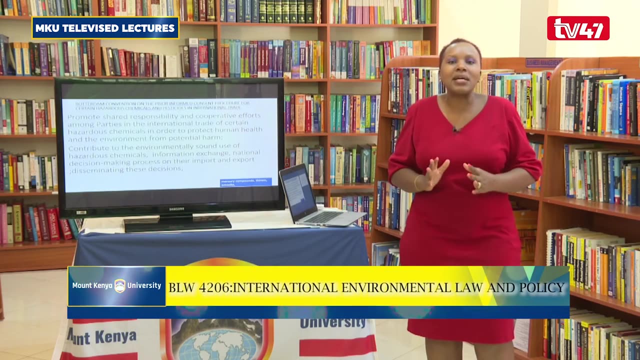 convention talks about. you got rwanda sharing information with us, kenya accepting that the goods, that the hazardous substance is going to be disposed of in our country, but because that the products will be transiting and moving through rwanda, rwanda also must get consent, must consent. 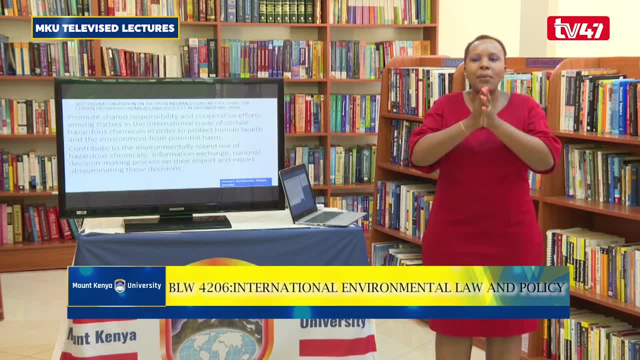 that i, as a country, as the president, paul kigame, i agree that the product which is leaving my country is going to pass through uganda and uganda, as the president, his excellence in 70, agrees that uganda is going to be a transit zone and kenya agrees that the worst product will be. 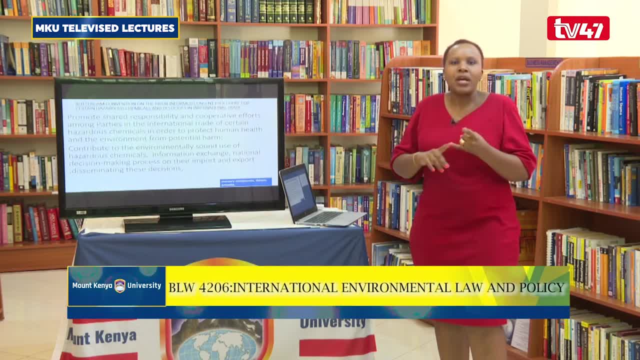 dumped in kenya. so the constant level is threefold. the exporter must consent and give prior proper information on what is transporting, giving details, giving the on the chemical that's transporting, the capacity, the concentration level and, in the event of a leakage, what measures does uganda? 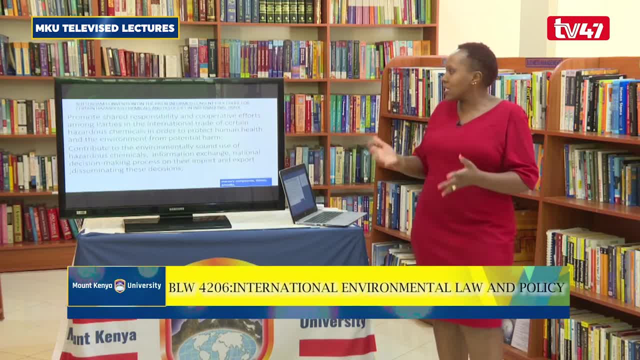 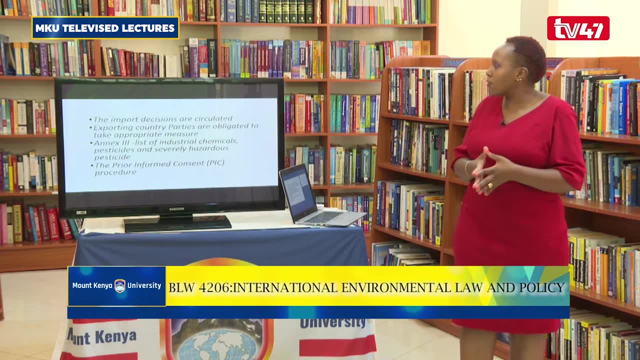 as a transit country, is able to take in terms of management of these hazardous substances. so one of the things that in just got detailed in terms of the rotterdam convention is it talks about the import decisions are circulated, remember, if there are three countries- uganda, kenya. 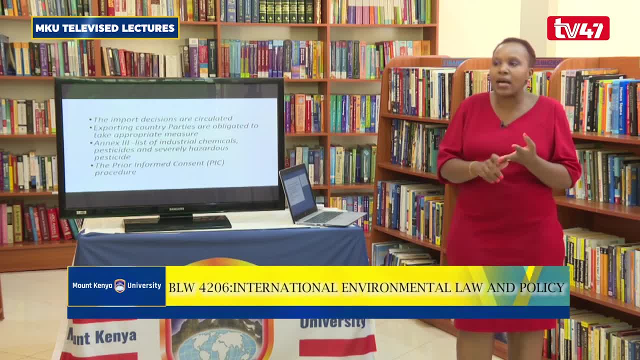 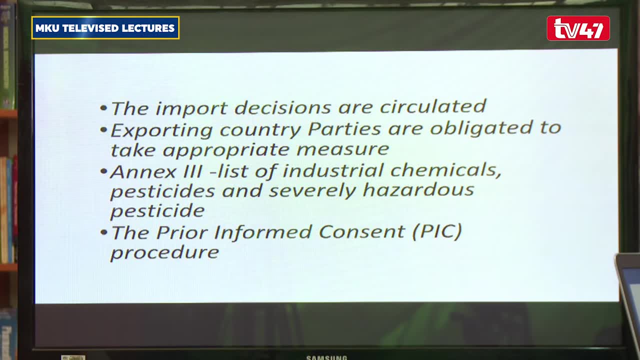 and tanzania. uganda, no uganda. rwanda and kenya. the business is between rwanda and kenya, but the decision must be circulated in east africa generally. that late tanzania let somali, let burundi know there's a transaction of international movement of azadiah substances between rwanda and 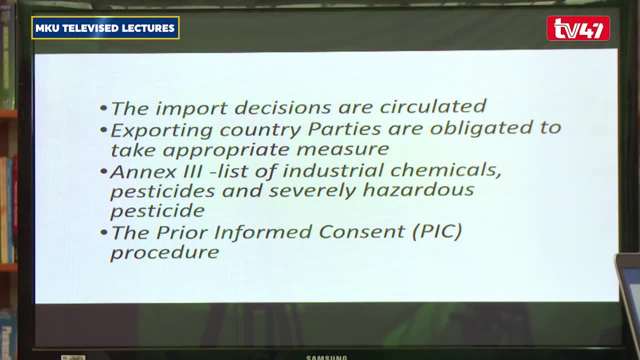 kenya so that, in the event of exposure, all the countries in east africa must be aware of it. remember again: this is a discussion that must begin at the global level through the conference of parties. we've been discussing about the conference of parties as a decision-making body. 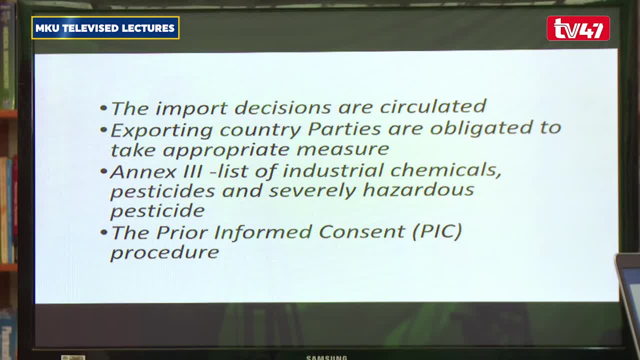 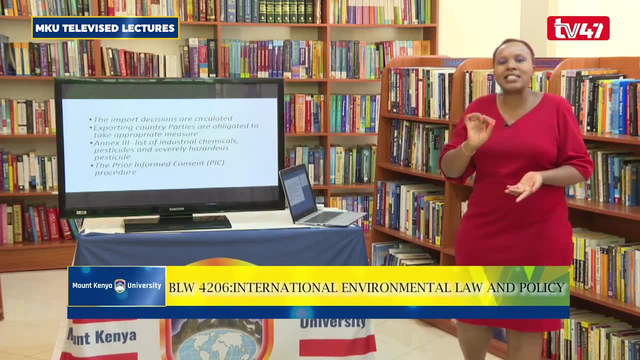 at the global level. so the decision again must be communicated to the conference of parties. so the convention, rotterdam convention, insists on informed consent that is circulated and disseminated within all the concern parties and at the global level. the other thing is, The third one is exporting countries are obliged to take appropriate measures. 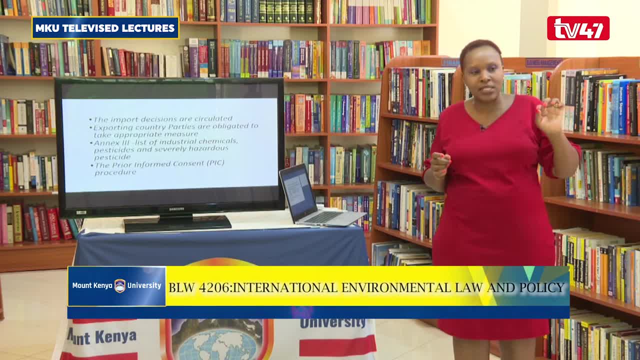 This takes us back to the other class on principles of international environmental law. Precautionary principle, preventative principle, Polluter pays also comes into play. Compensation also is one of the principles that, if at all, there's a leakage because of improper packaging of these hazardous substances. 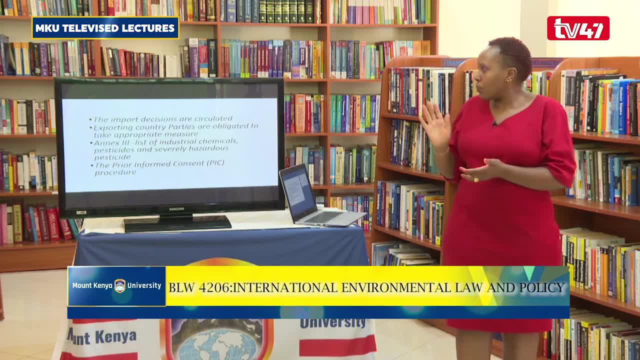 the exporter country is liable in terms of the management of that product. So the owner will be in Rwanda. The owners for taking care of precautionary principle, preventative principle, before the goods is released is basically in Rwanda, before the goods transit through Uganda and comes to Kenya. 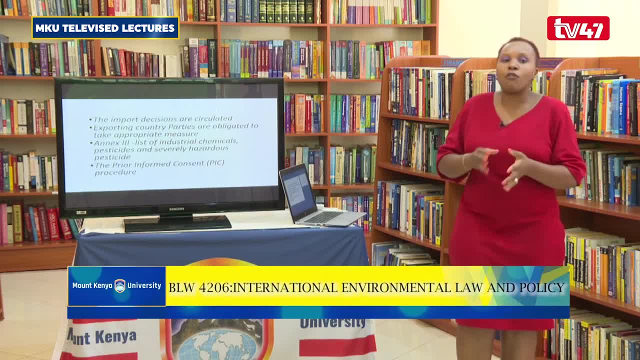 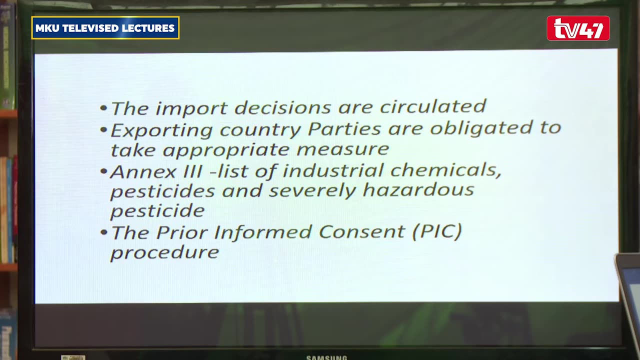 The Rotterdam Convention also talks about annexures of list of pesticides and chemical substances that are extremely dangerous, So that if a country decides to trade in these chemicals which are listed in annexure 3, which are severe, Severely hazardous pesticides, they have to again consent. 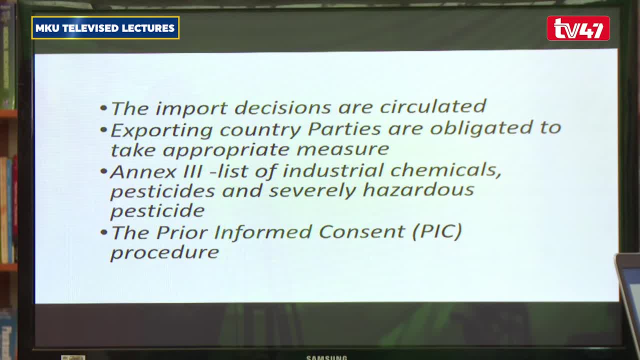 That I have not only consented to that trade of hazardous substances, but also, in addition, I have consented in the trade of severely hazardous pesticides that are listed under annexure 3 of the Rotterdam Convention. So it goes deeper. There's a deeper conversation on the prior informed consent. 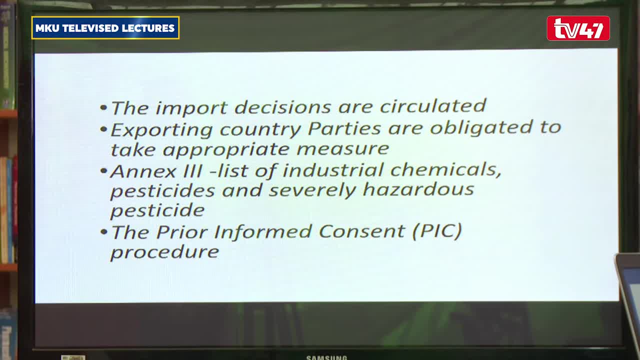 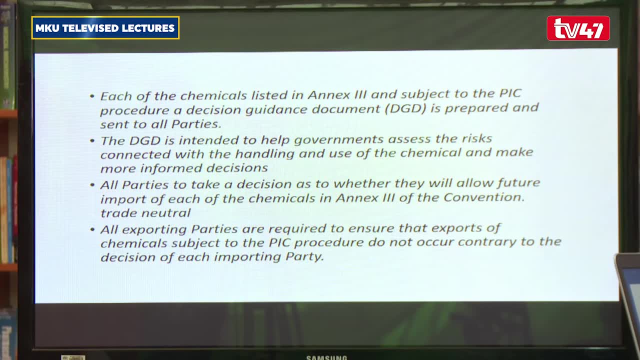 which is basically the PAC procedure, which is the main fundamental principle that is introduced in the Rotterdam Convention. Then the Convention also introduces a committee. It's called the Chemical Review Committee. This committee is basically the one that helps us to review annexure 3.. 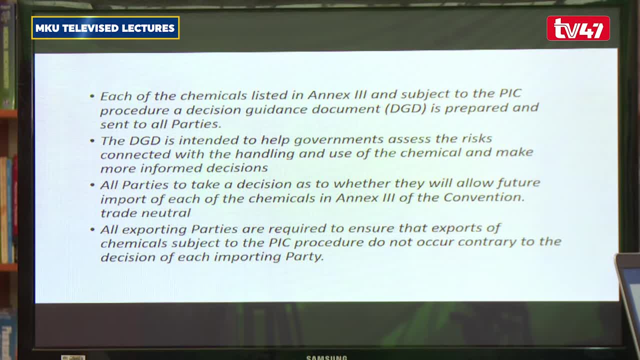 That which chemicals have now been clustered in 2020 as most severely hazardous substances. So it keeps on reviewing the annexures to be able for countries to be informed on what are the new measures that they should be taking. We have also one of the procedures called the Decision Guide Document. 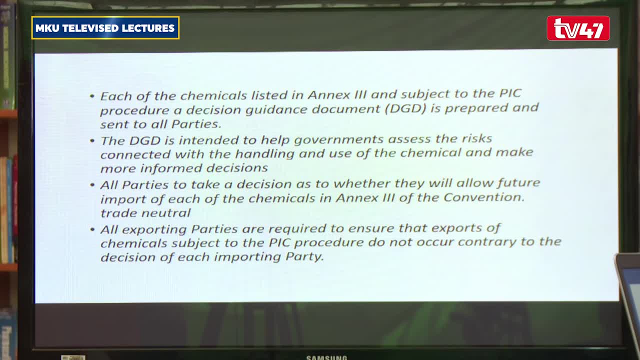 which is prepared and sent to all parties, Basically listing all the additives. Other annexure: the chemical documents, the chemicals that are listed under annexure 3.. So once it is updated it is shared via the Decision Guide Document. Then all parties must take a decision as to whether they will allow future import. 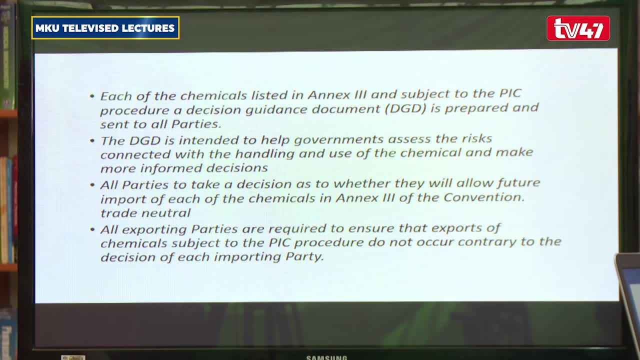 of each of the chemicals listed in annexure 3. So that we can decide to trade with Rwanda on one of the chemicals listed in annexure 3.. But we say: after our trade in 2020,, moving forward in 2021,. 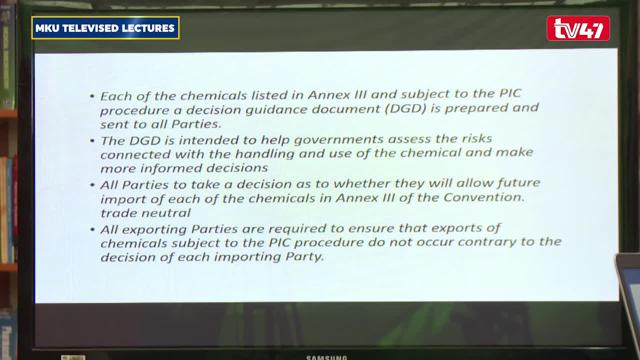 we will not be able to trade in any chemical that is listed in annexure 3. So that the global environment is aware of your decision. Another aspect is: all exporting parties are required to ensure that exports of chemical subject to their prior informed procedures do not occur contrary to the decision of importing parties. 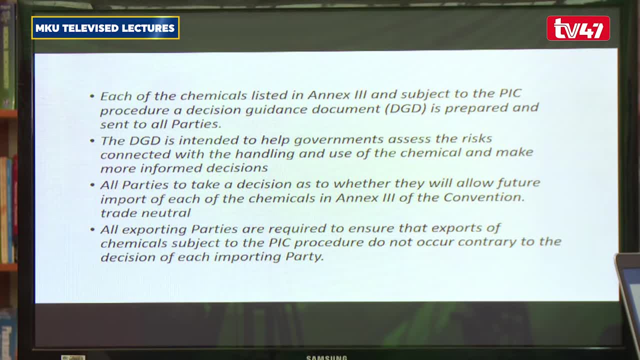 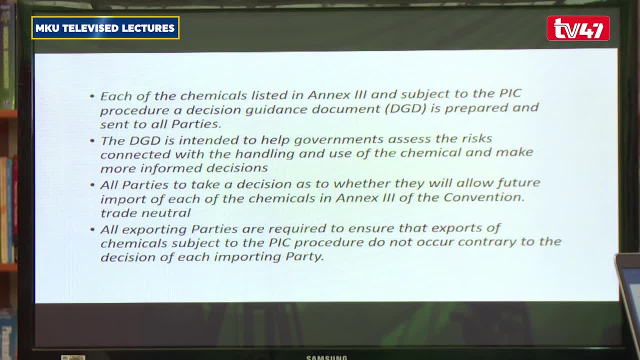 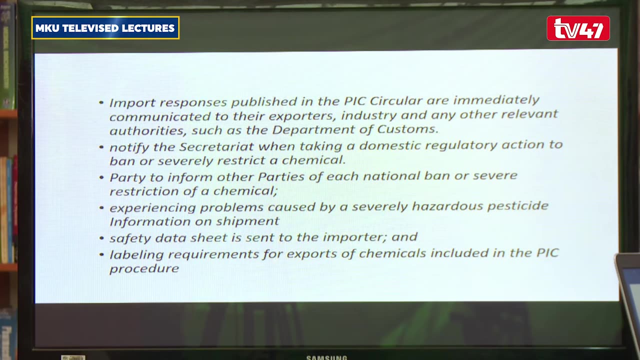 The exporting country must adhere to our consent, must adhere to our regulations, so that we don't have illegal dumping of waste products, as it happens in Haiti, it happened one time in Nigeria and many other developing countries. So, basically, you need to notify the Secretariat. 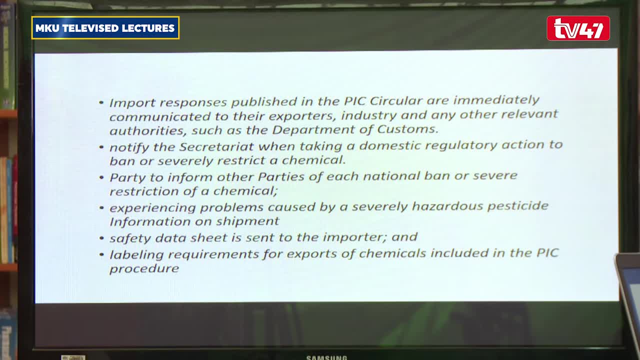 Secretariat is basically the UN environment- on the domestic regulatory actions that a country has taken, Whether you've banned the transportation or whether you intend to do trade with a country on transportation, On transportation of those hazardous substances, Then you're also supposed to share your experience. 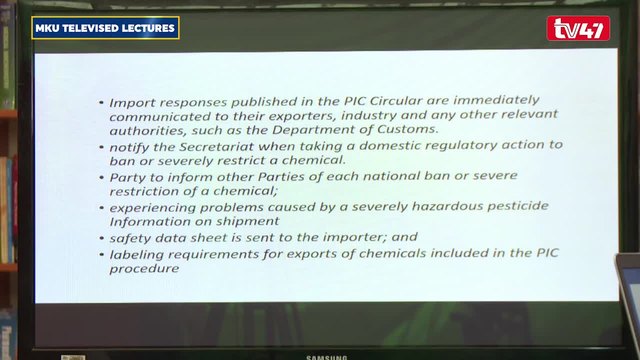 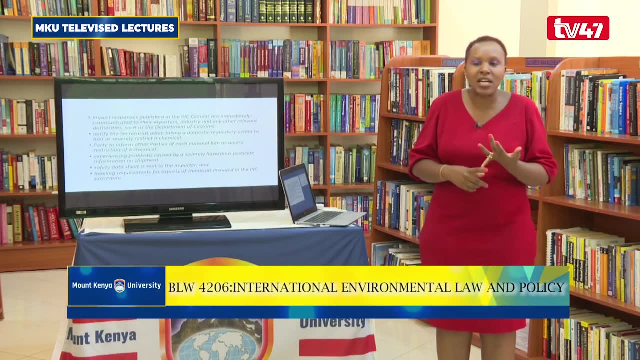 After we've done trade with Uganda, with Rwanda, and we experienced challenges in terms of management of these products. They are, yes, dumped in our country, but our management infrastructure, resources, human resource was not sufficient enough for us to be able to manage these products. 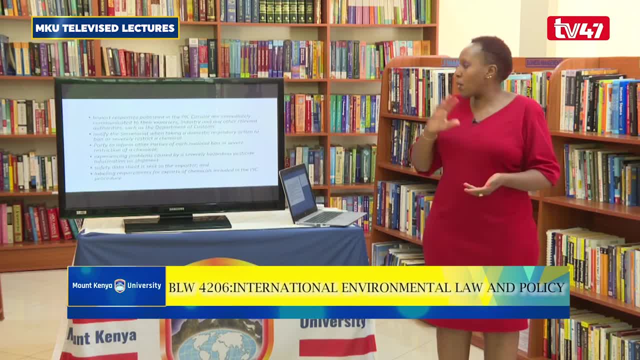 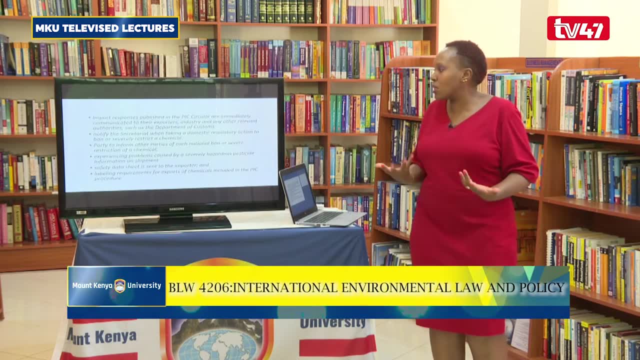 We must be able to communicate back to the exporting country, must be able to communicate back to the UN environment and the Secretariat, basically on what are the challenges that we experience and what measures can the global environment develop in dealing with that. It also introduces safety data sheets to be sent to importers. 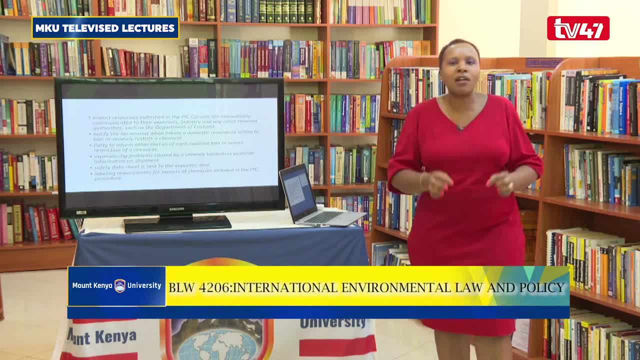 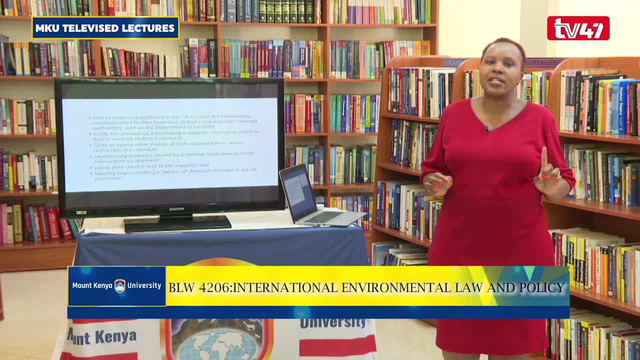 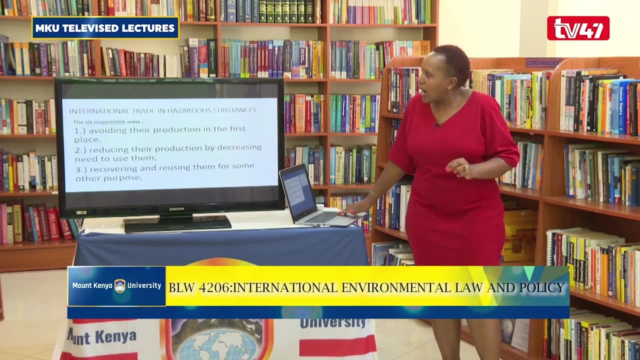 to be assured that you understand the risk involved in importation and trade in those substances So that in future don't say we did not understand the risk, It will not be tolerated. You must be able to sign the data sheet that explains the challenges. 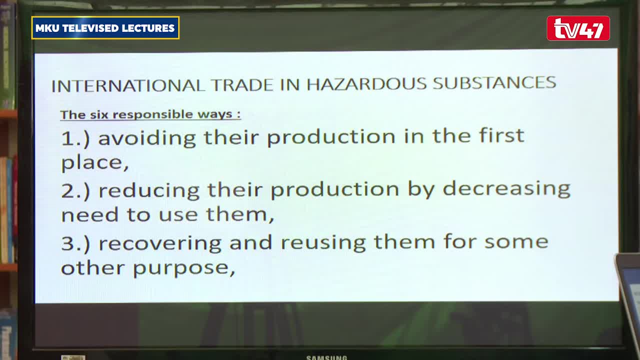 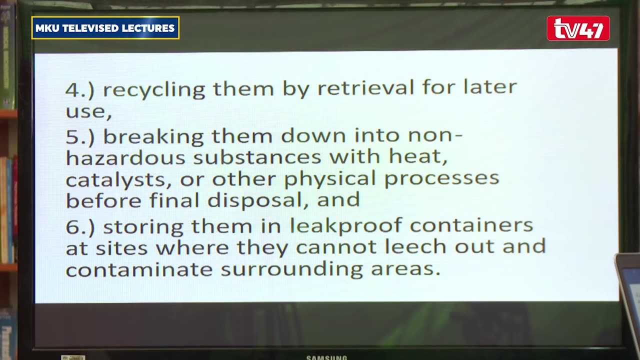 There are six responsible ways of doing it. Avoiding their production in the first place is recommended, Then reducing their production by decreasing need to use them, And then recovering and reusing them for some other purposes, basically recycling these products. Then we're also advised to break down some of these products so that they're not toxic. 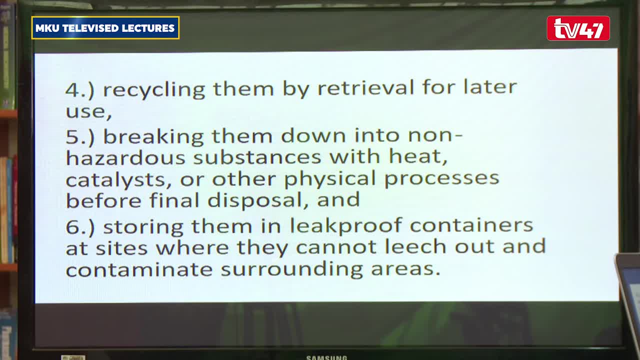 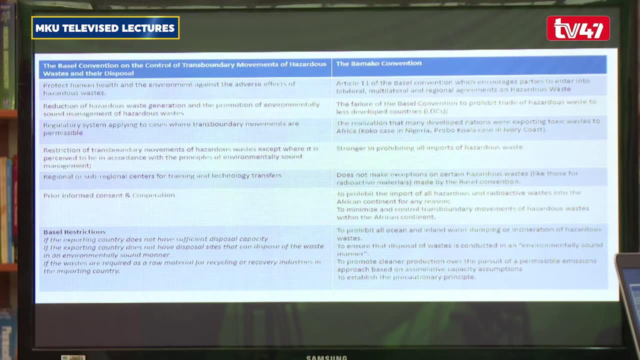 Removing the different components of a product so that when they- because when they're mixed, they become more dangerous and severely toxic, Then storing them in a lock-proof container. This is basically the things that we recommend countries to develop Beyond the Rotterdam Declaration. 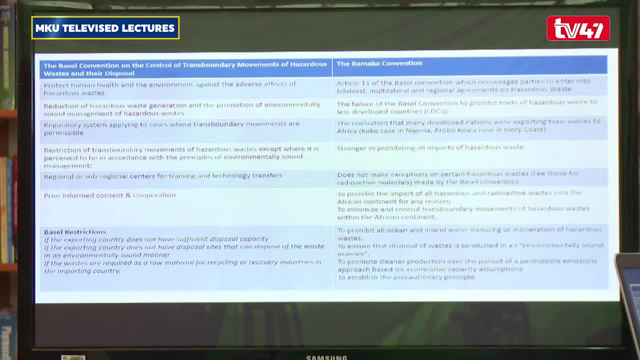 beyond the Rotterdam Convention, we have two additional conventions. One is called the Basel Convention on Control of Transboundary Movement. From the title, it is the control of transboundary movement of Azadea's waste and disposal products. The other one is the Bamako Convention. 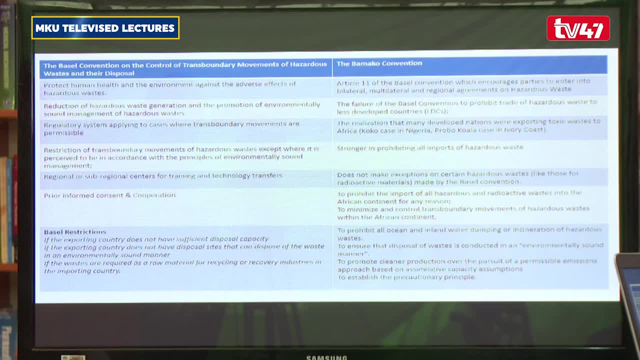 Bamako is basically African-based. It's an original treaty. It's an original treaty that looks at the movement of hazardous and toxic substances within Africa and also the movement from developed countries to developing countries, of which most of them are in Africa. So, basically, the Basel Convention talks about the need to protect human environment. 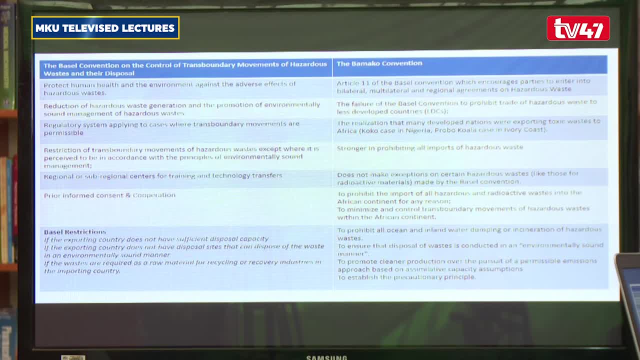 It talks about reduction of Azadea's waste generation of these products. How can we be able to reduce these products, And one of the things that it has copied and replicated in the Rotterdam discussion is prior informed consent and cooperation is one of the things that is provided for in the Basel Convention. 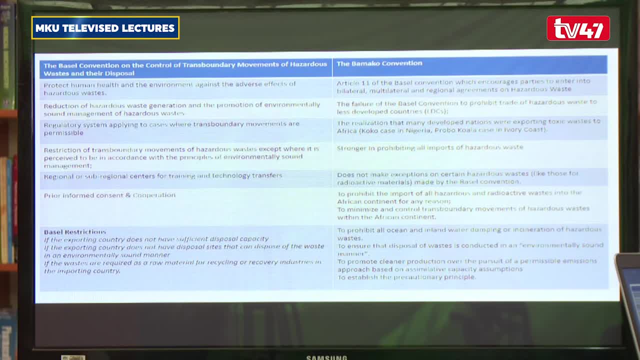 And the critical component of this convention is the restriction that it brings aboard, That if the exporting country does not have sufficient disposal capacity, you don't have a ship, you don't have a tank, you don't have a container to dispose of these products. 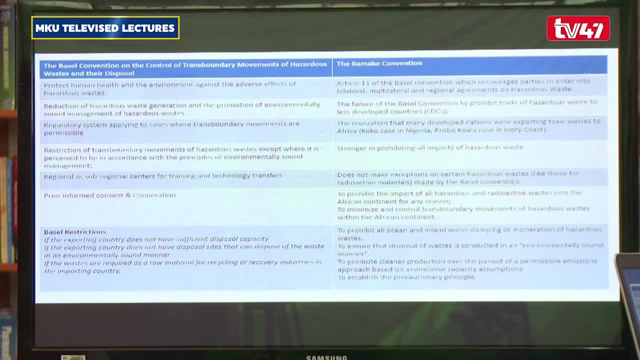 to export of these products. do not engage If the exporting country does not have disposal sites that can dispose of waste products that you want to export. but you've not identified a country where you're disposing of. if it is Kenya, you've not identified. maybe it's Uganda, it's Tanzania. 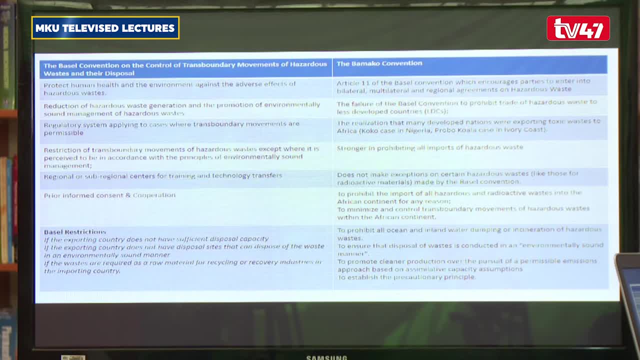 you will be restricted to export your product. The other restriction is if the wastes are required as raw materials or recycle recovery industry is the reporting country that these materials that you're trading in must be something that is, must be something that is useful to the country. 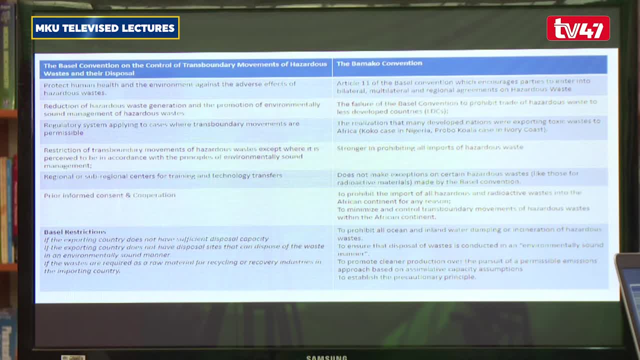 So that you don't just trade with materials, that you're going to dump and sink them, but you want to see how these materials can be recycled by different countries to be able to be used as a product to produce something useful for the country. The Mabako Convention, the thing, and one important aspect of it. 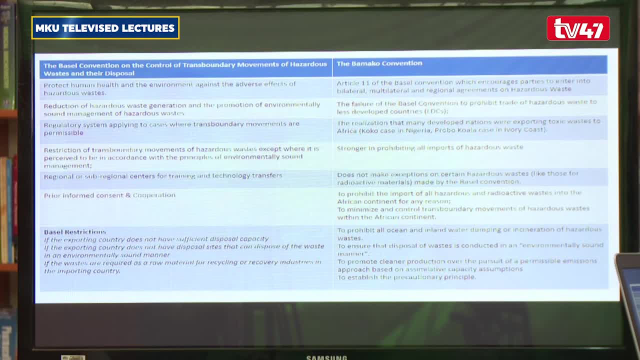 is that it introduces the limits, the transboundary movement of radioactive materials, which the Basel Convention failed to do. Basel listed a number of chemicals and hazardous toxic substances and excluded radioactive materials which we know. in most developed countries, the radioactive materials are the most byproducts of industrialization. 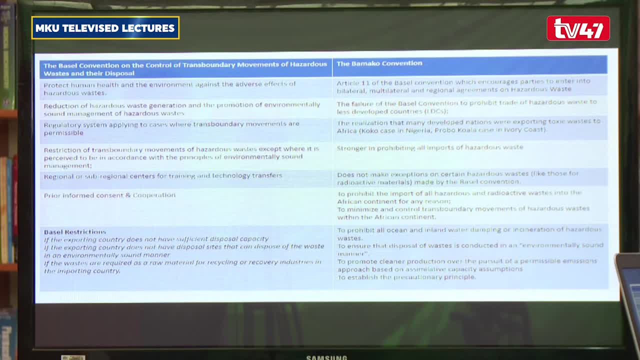 So the Mabako Convention came on board and introduced that aspect and said, as part of the next step of the chemicals we're dealing with, it's important also to look at the radioactive materials and restrict the movement of these radioactive materials in the list. 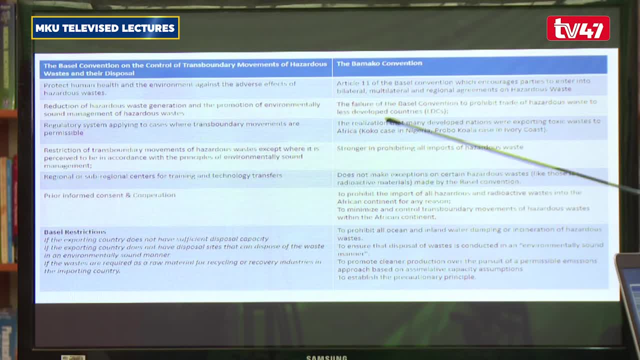 developed countries. The emphasis is on least developed countries because we know industrialization happened mostly in developed countries, But also we know that within Africa we have countries that are developed, like South Africa, Nigeria, even Kenya ourselves. So we also want to limit transboundary movement of these hazardous and toxic substances. 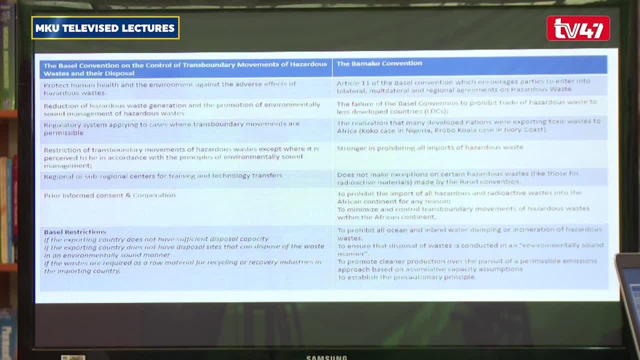 within Africa as a whole. So this is why we needed a convention specifically to speak to our needs in Africa, To lead to speak to our challenges in Africa. So that's the most important part of this convention. Of course, it prohibits dumping at sea level. 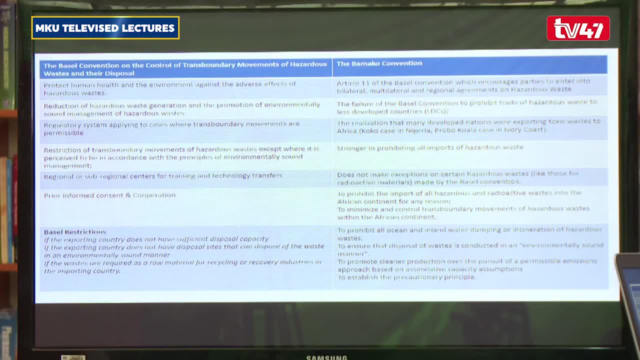 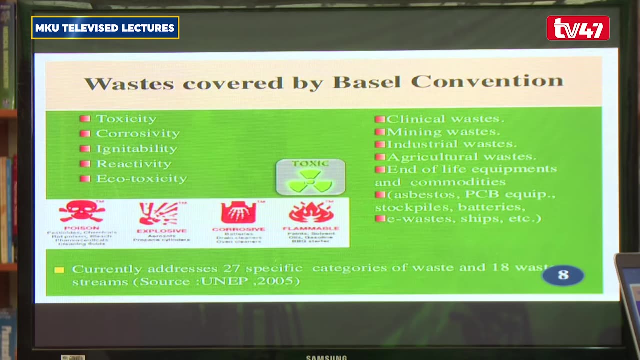 dumping in inland waters. Remember the Basel Convention talks about dumping at sea. But we recognize in Africa we may not have connectivity to many seas but we have inland waters and lakes, so that we also prohibit dumping at that level. This is just a slideshow on some of the waste products. 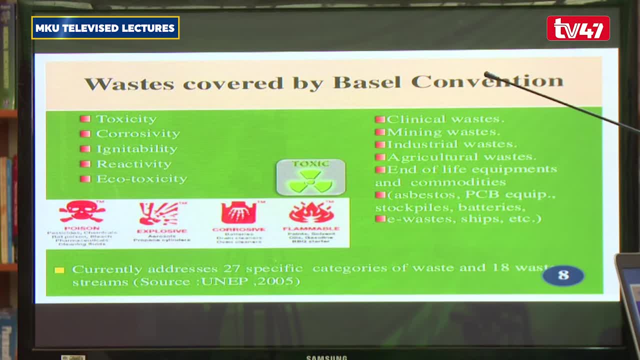 You have them from clinical waste. In hospital you find injection being put separately, Cotton pads being dumped separately. We have mining waste, industrial waste, agricultural waste. We have e-waste ships also dumping at sea level. Those are some of the examples. 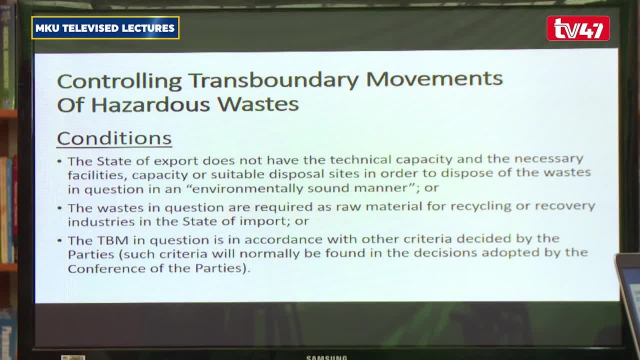 Then, in terms of our control, we have conditions, which we've also discussed. What are the conditions that must be met in terms of transboundary movement of these products? It's also part of the discussion that we've been talking about. So the next item. 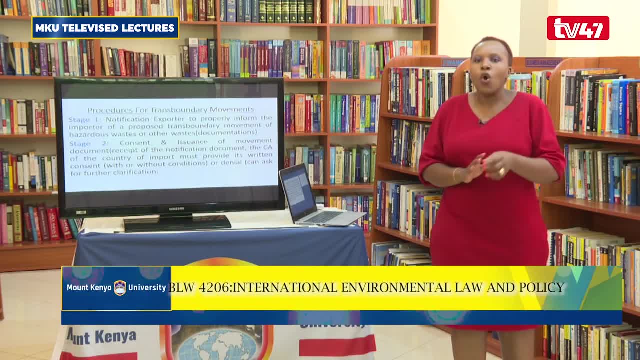 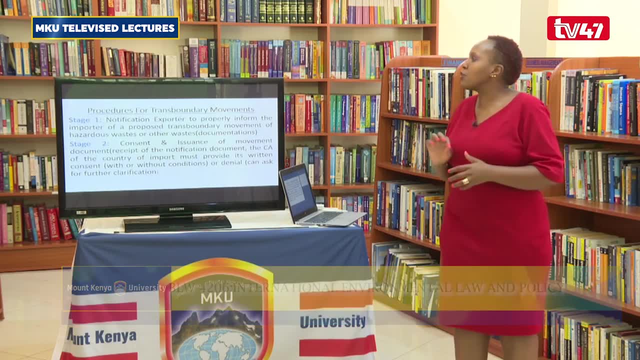 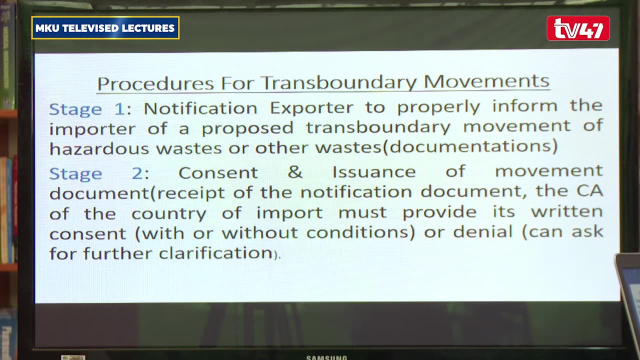 we want us to look at the procedures for transboundary movement, which is the concluding remarks for our presentation for today- That countries must give notification, proper documented notification, signed by the relevant authority, If it is NEMA in our context, if it is the custom duty in our context. 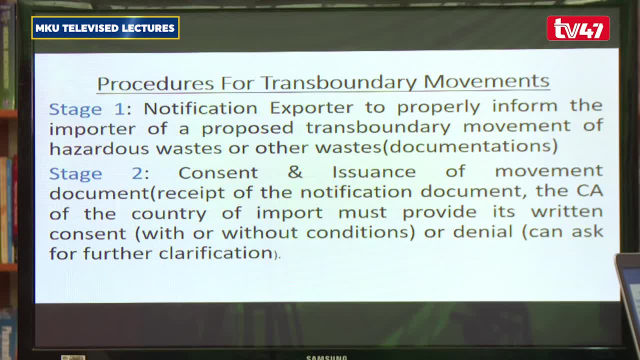 KRA must be involved. All the relevant institutions within their country must prove that they got the notification from Rwanda that they intend to dump their waste in Kenya. Then we must have consent. The prior informed consent also is a documentation, A number of different detailed documentations that are needed. 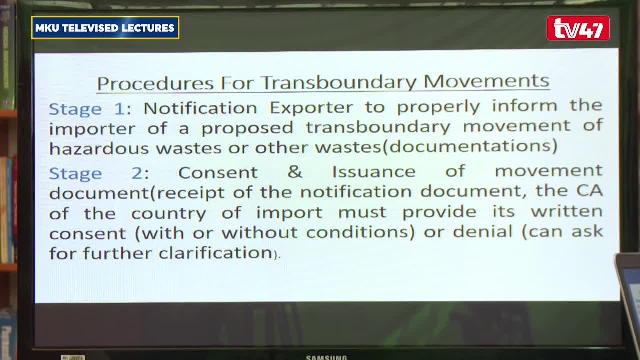 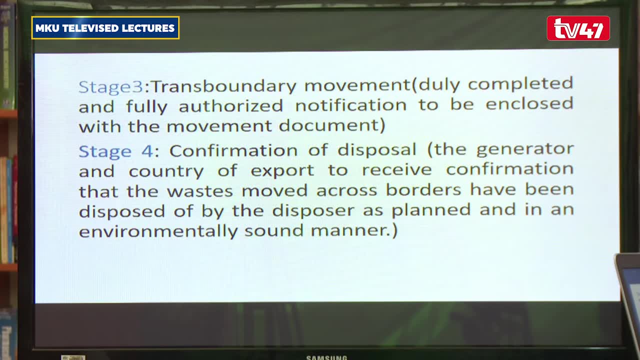 You must prove that you also received the consent. Consent must be circulated within the member states that are involved in the transaction. Stage three is the transboundary movement itself, So that the document must list down what countries they are passing through the details of that chemical that is being transported. 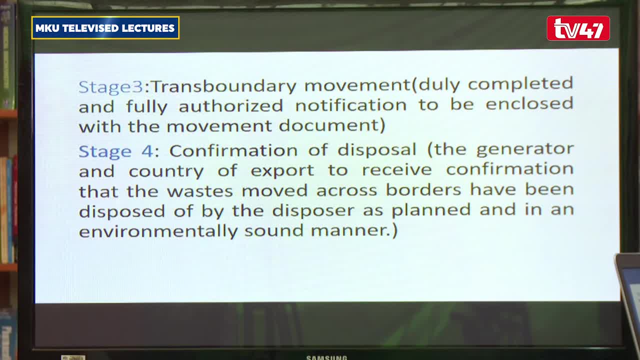 All the details must be provided in the document. It is a transboundary movement document. It is also a lot of paperwork. The last one is confirmation of disposal. Kenya must alert the other states that, yes, we received the goods on the 20th. 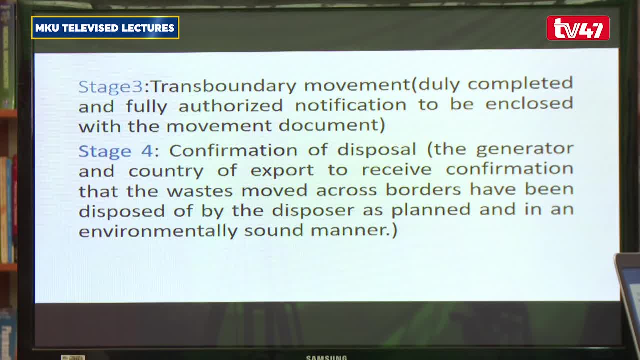 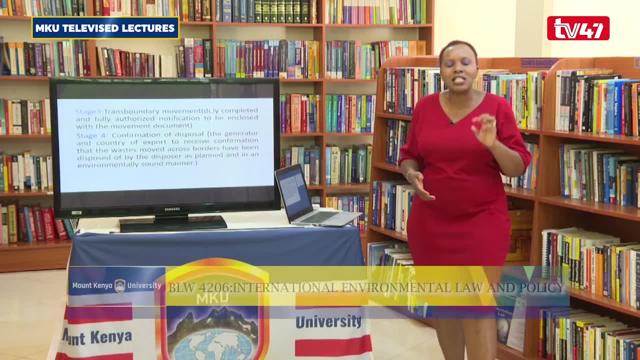 These are the goods that we received. This is how we intend to dispose of this product, Or this is how we intend to recycle this product within the country. So from today's discussion, emphasis is placed on the procedure for transboundary movement of these products. 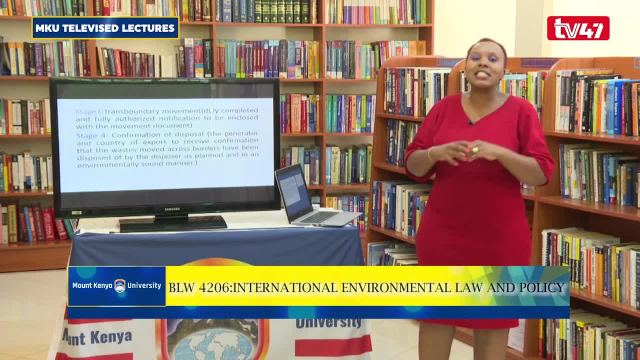 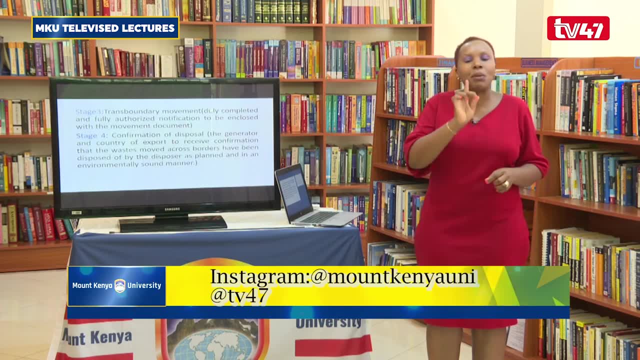 We've agreed at international level that it is important to do trade. It's okay, But there is caution. There is caution, There is restriction of this trade, But also there are conditions that must be met And the procedure is the four stages that we've discussed. 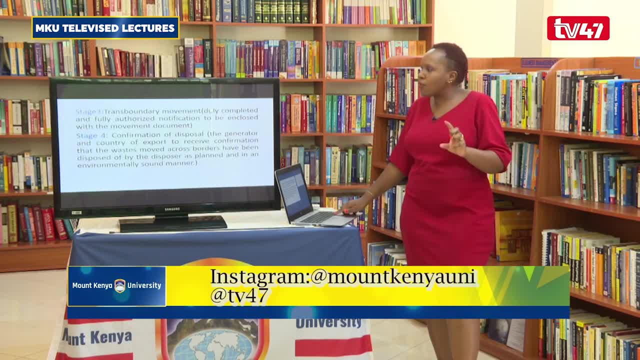 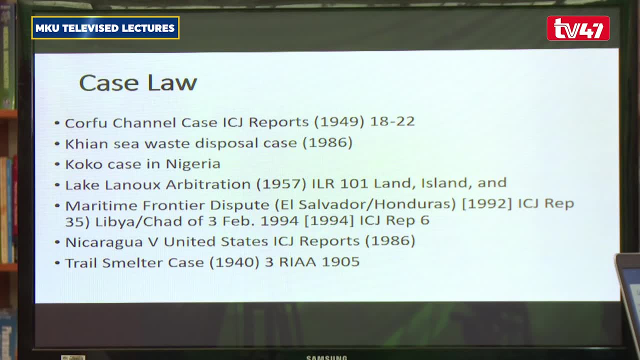 As a takeaway, the four stages are very critical in terms of transboundary movement and the relevant laws that we've discussed. There are a number of case laws I want to attract you into reading so that it's only not one way. So please find time to read the Kofu Channel case. 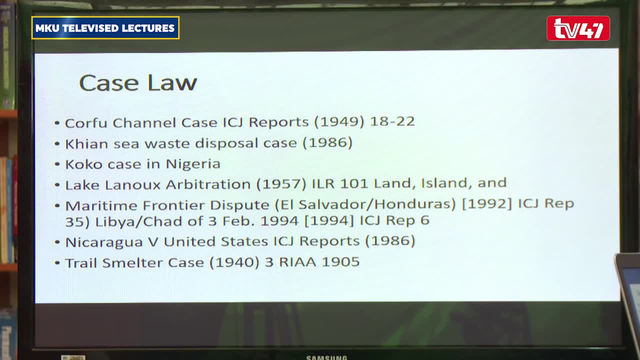 Read the KNKC disposal that happened in Haiti, The Koko case in Nigeria- Those top three cases will be able to give you a summary of what it means to dump. What is the implication to the health of human beings and the environment in terms of dumping products? 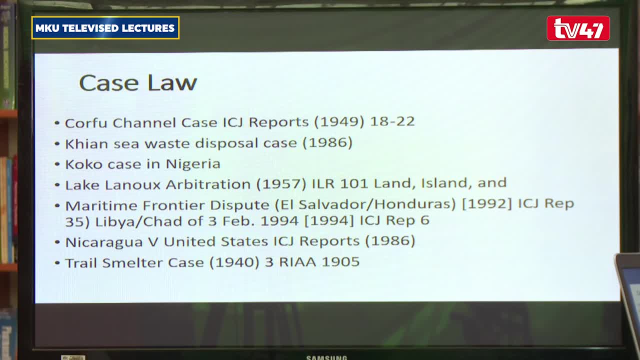 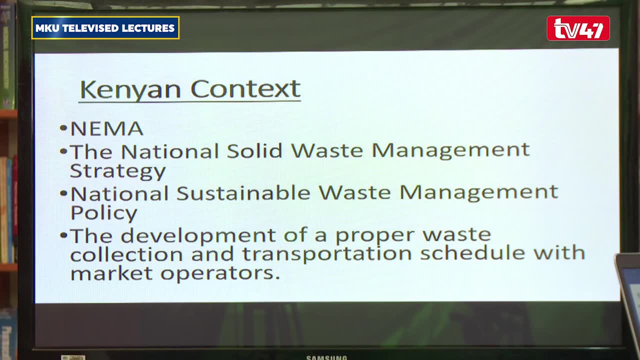 at illegal dumping of products without prior consent, prior notification and approvals. Kenyan context: we have a number of legislation. We have the National Environmental Management Authority. We have the National Solid Waste Management Strategy and Authority within NEMA- A number of legislation that you've come up on board. 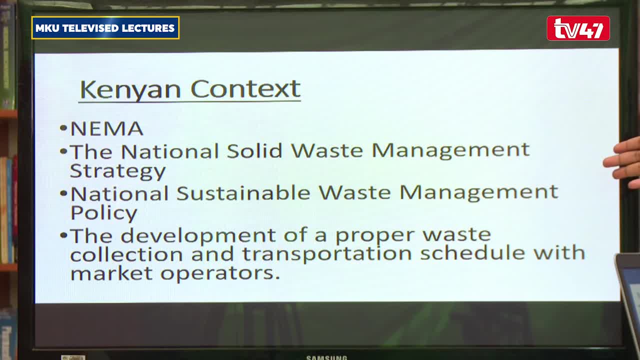 with as an institutional, as a country, to be able to manage waste product. The challenge is still there: What do we do with Dandora? Who will manage Dandora? It's one of the products that is exposing the citizens, who have hazardous and toxic substances. 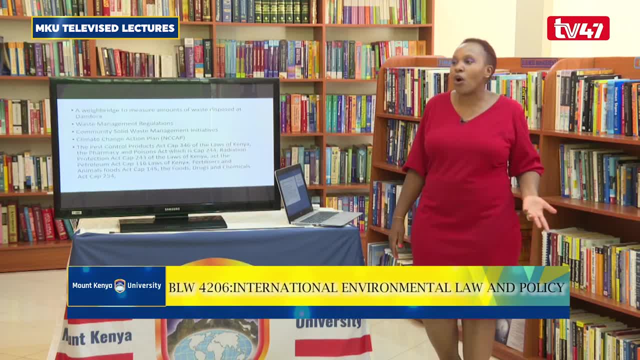 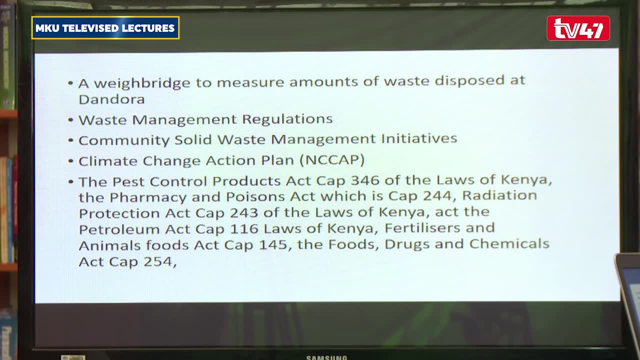 But as a country, what are we doing about it? It's a challenge for all of us, Challenge to the state, Challenge at the global level. Help us, if you can, in terms of coming up with a plan to be able to manage the waste product. 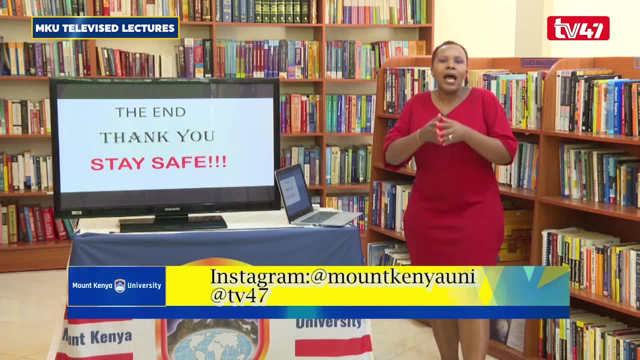 I've come to the end and thank you so much for listening And I encourage you also to have conversation on the legality on the use and threat to use of nuclear energy. Please refer to the advisory opinion by the ICJ. Refer to the advisory opinion by the Security Council. 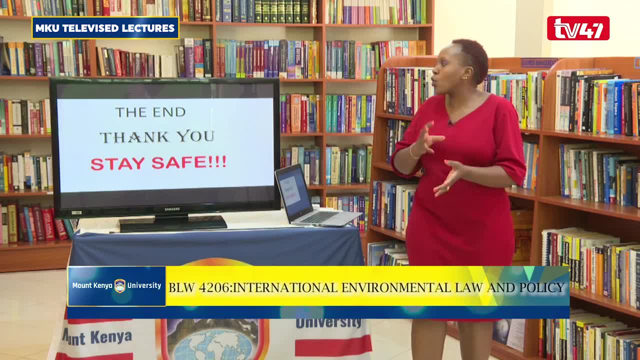 of the United Nations. It will give you an outlook on whether it is legal or illegal to use nuclear weapon and nuclear energy. Please, let us catch up on the e-platform for further discussion. Let us continue to have our chat. Let us continue to have in our conversation.